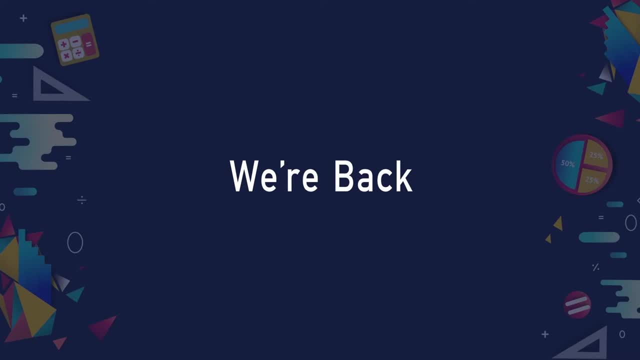 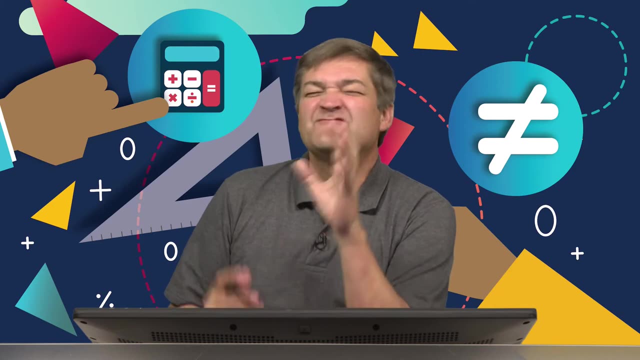 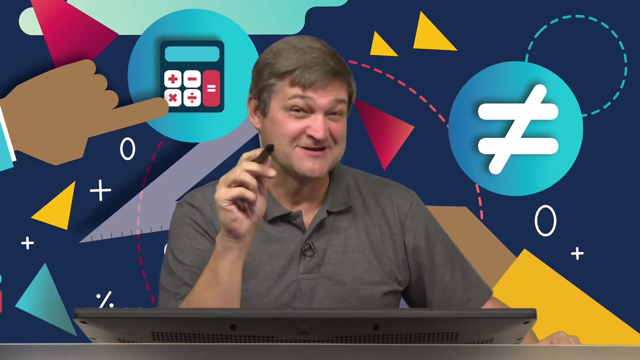 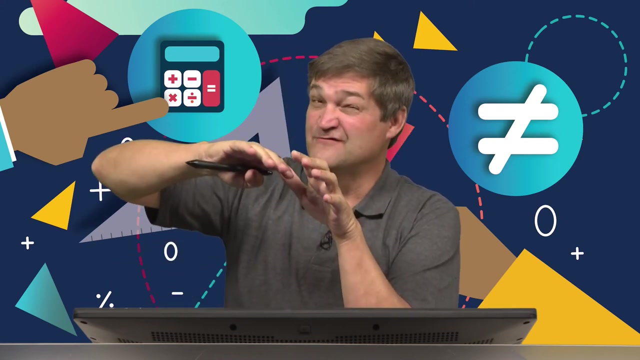 It's my wife's birthday soon and I've got a fantastic plan for her birthday present: I'm going to take her on a holiday. Yep, that's right, We live in Joburg. We're going to catch the train, go overnight train, so we're going to have a little bed and sleep in it. 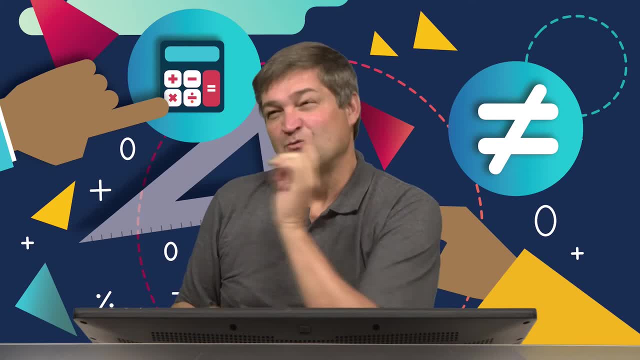 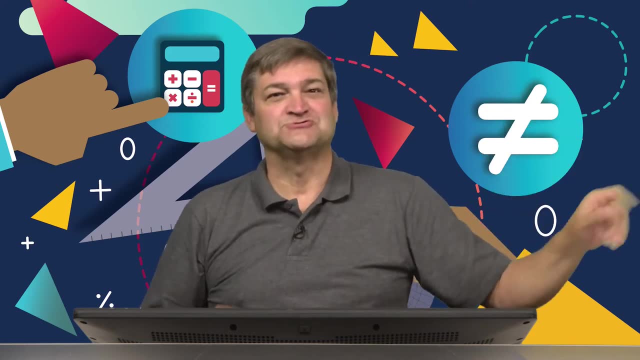 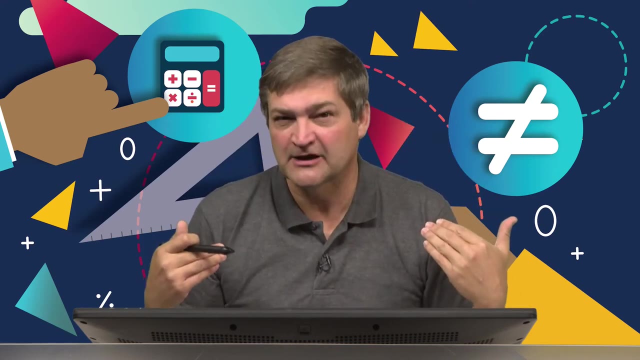 go overnight to Cape Town. When we get to Cape Town we're going to stay in Cape Town for two or three days and then we're going to fly back to Joburg. That is such a cool present and the best thing about that present is I share it because I go with her. That's a clever present, I'll tell. 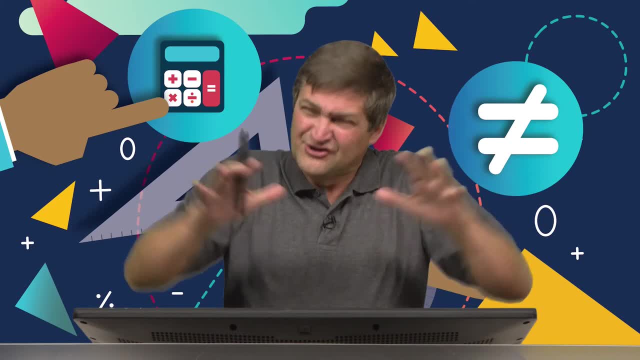 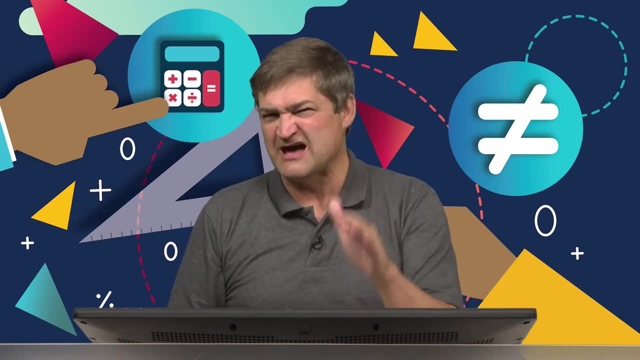 you what. But before I look at all of that, I've actually got to say, hey, this is going to cost me a lot of money, So I'm going to have to look at all the money that I have coming into my bank. 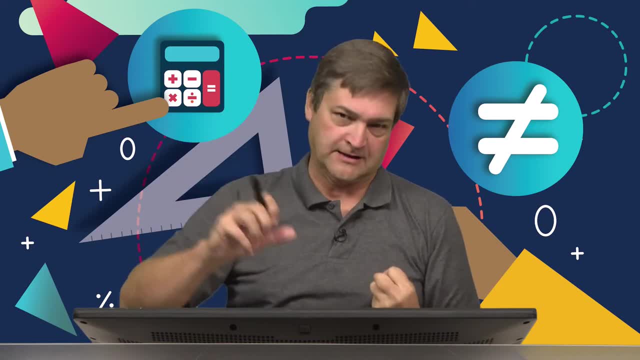 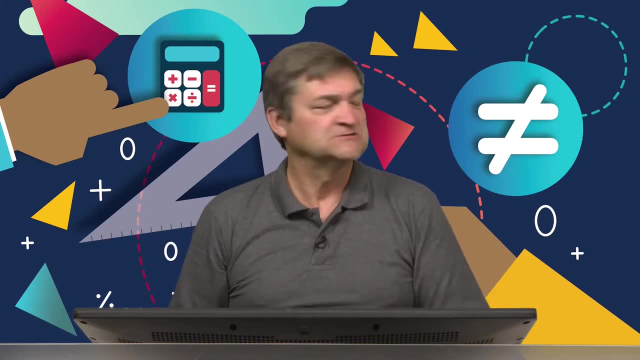 account and all the money that goes out of my bank account to see how much I've got left over, to see whether I can actually buy her this present. In fact, I shouldn't talk so loud because she might be around and hear this, So I've got to talk a little softer here. 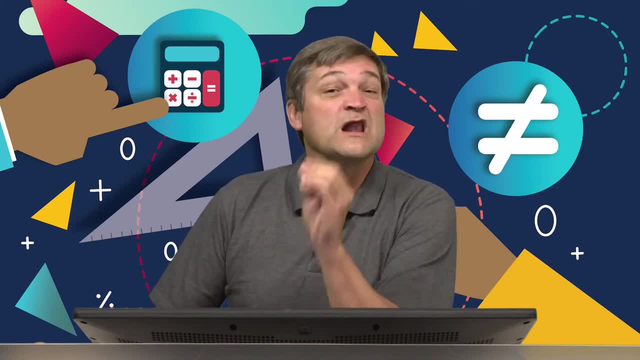 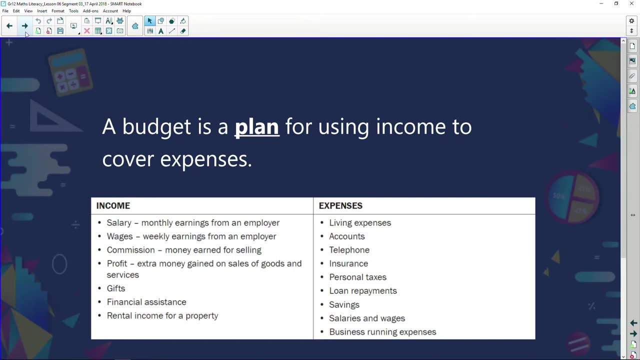 But that's the idea. Will I have enough money to buy her that present? Let's have a look here. A budget is a plan for using income to cover expenses. In other words, do I have enough money to cover my expenses? Let's have a look at some of the. 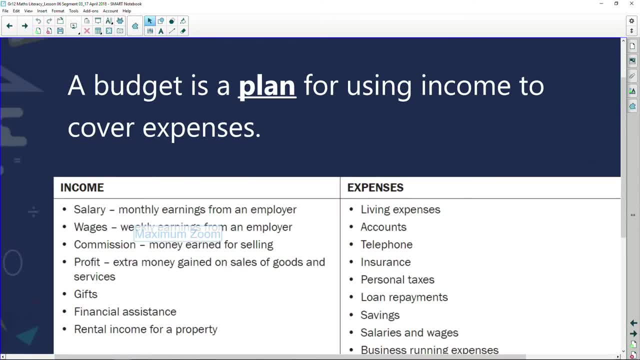 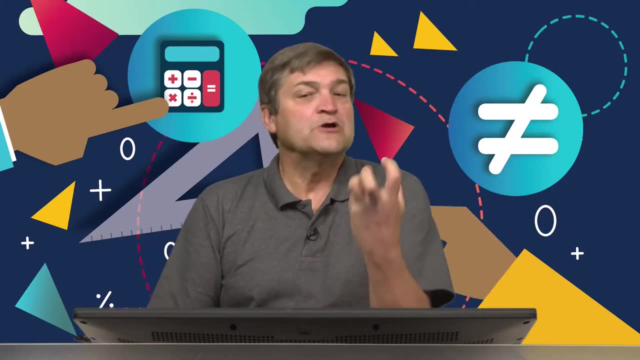 income and some of the expenses. All right. So income Income is like a salary: monthly earnings from an employer. Wages are weekly earnings coming from an employer. So you could be paid monthly and we call that a salary, or you could be paid weekly and we call 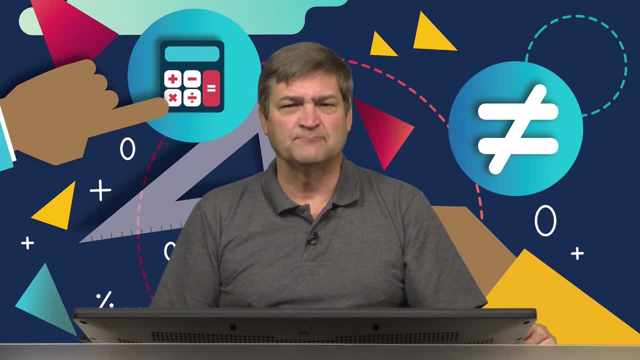 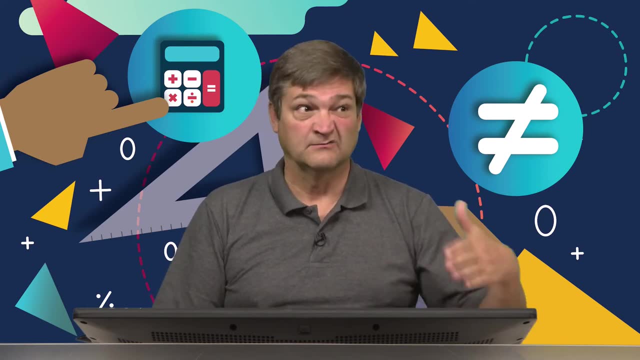 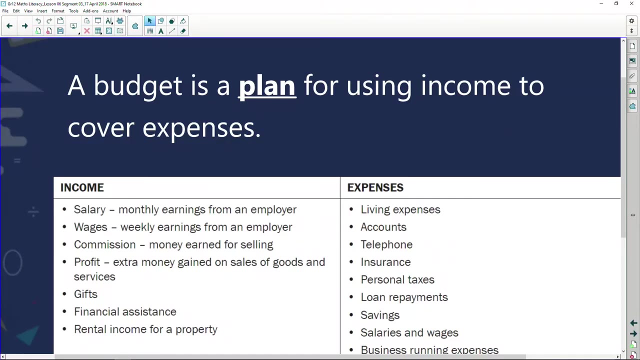 that wages. Okay. I always say to my boss: I'm paid very weekly, Okay, Like hardly anything right, Very weekly, but not like Monday to Friday, just like week. Okay, Bad joke, bad joke. Then we can also get income from commission. In other words, how much money am I earning? 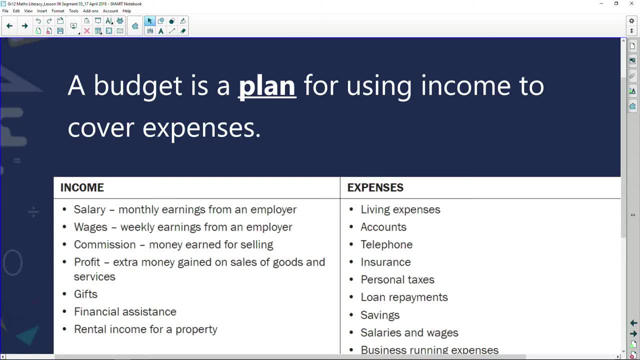 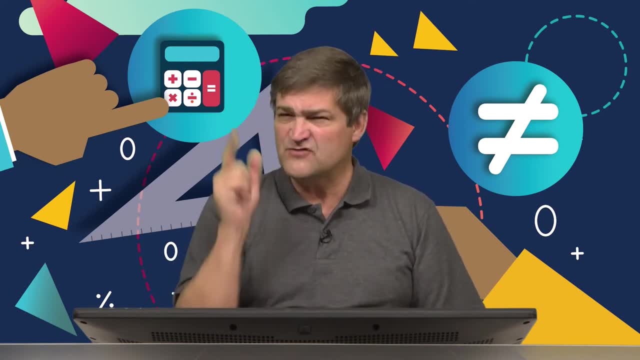 from salary. I'm selling things. So if I were to be a car dealer and I'm selling cars, you need to understand that my boss could come to me and say: you know what? I will give you 10%. Every car you sell, I will give you 10% of the value of that car. If I sell lots of cars, 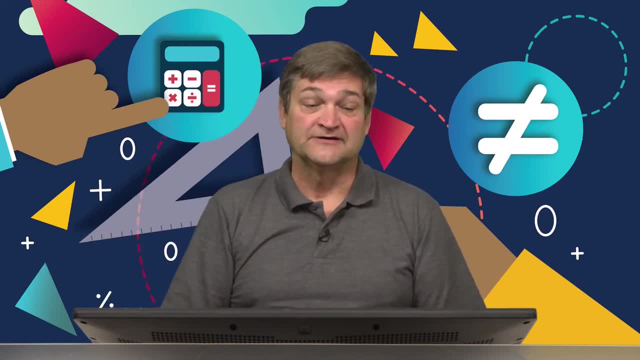 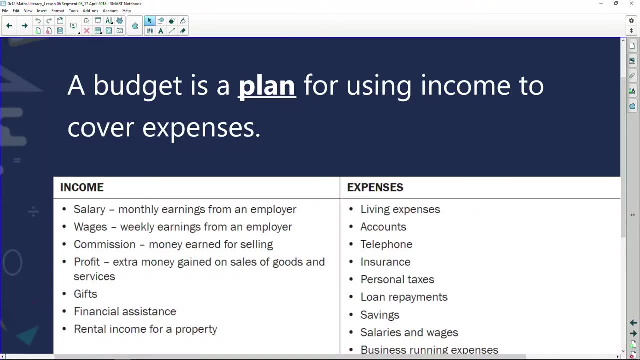 that month. fantastic, I'm going to earn a lot of money. If I don't sell a lot of cars, I'm not going to earn a lot of money right. Then we get profit and that's extra money gained on sales of goods and services. 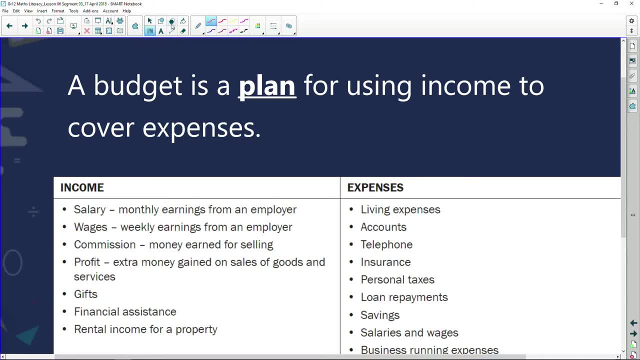 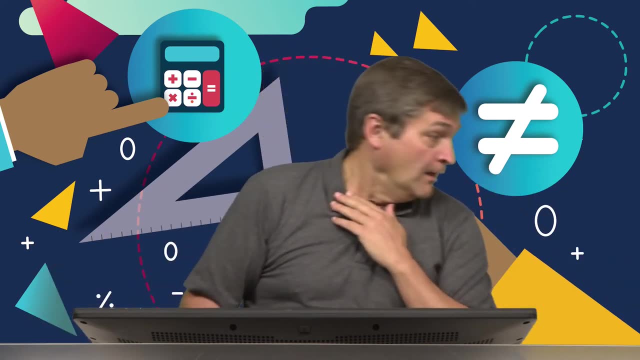 We might even land up with some fees or gifts, rather, where someone suddenly says: you know what? It's your birthday, Happy birthday. I'm going to give you a thousand Rand Like hey, cool, That's money coming in Financial assistance. Someone could be saying: you know? 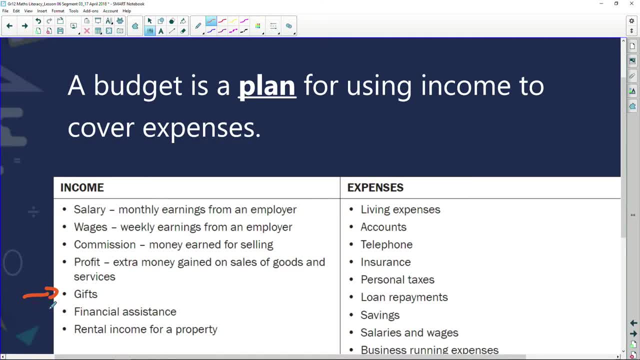 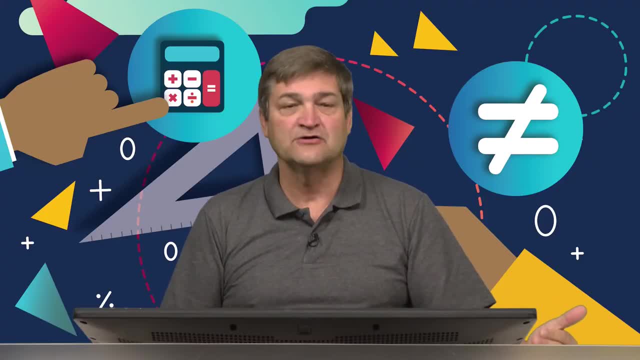 what This poor guy is battling. He's like: poor guy, Let's give him some extra money every month. All right, So you might have a few dollars. You might have a few dollars. You might have a family member, for example, and you know they're not earning very much. 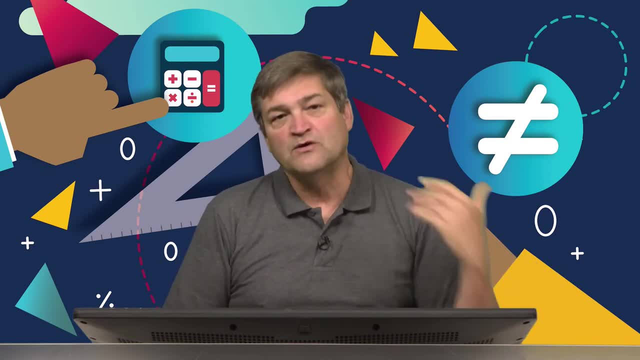 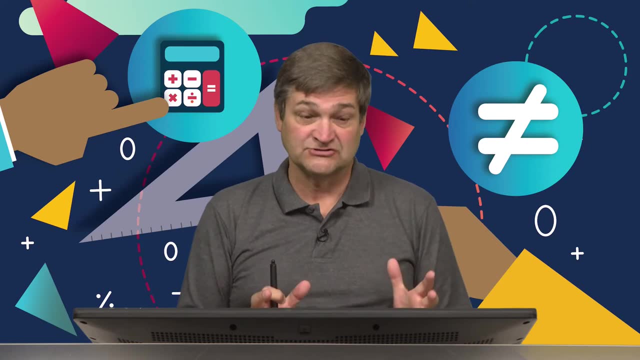 money And you decide you know what You want to help them out. You want to give them some extra money, So you're going to give them an extra 500 Rand every month. They see that as financial assistance and it's money coming in for them. 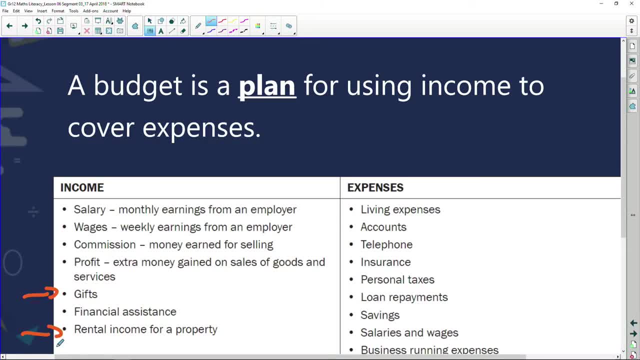 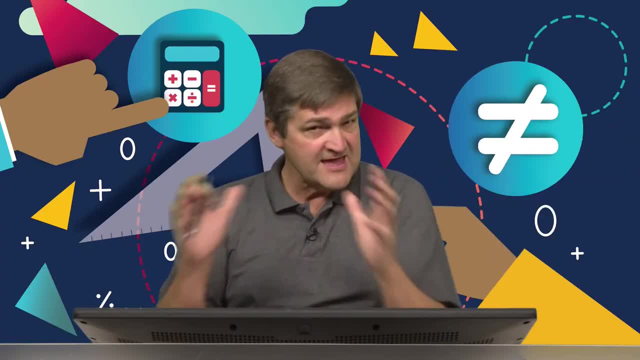 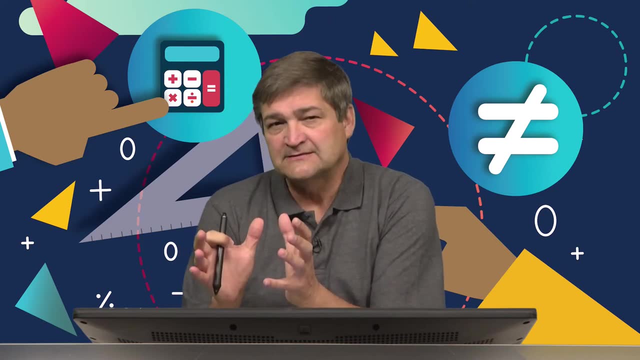 You might even get rental income for a property. So let's say you got a house but you're not living in it because you've got another house that you're living in That extra house they say you've got, or extra little bit of property That could be bringing you in some money. 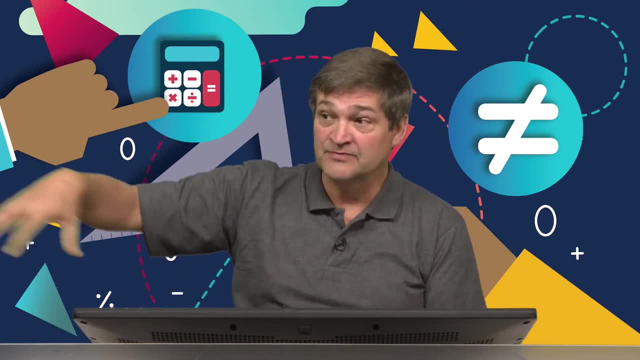 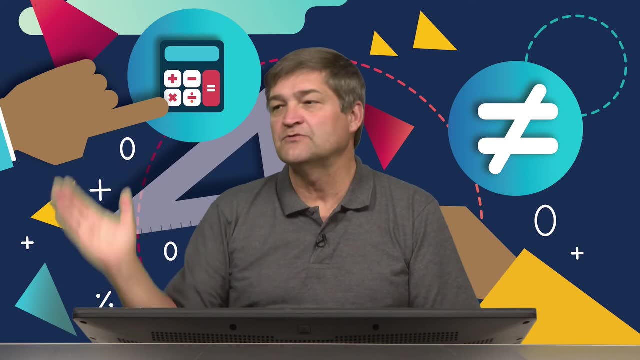 Maybe you've got a house and outside you've got a little hut area and you're wanting to rent it out, or a little chalet You're wanting to rent it out. Somebody comes and stays in and says we'll give you 2000 Rand a month if we can live in your little back gardens. 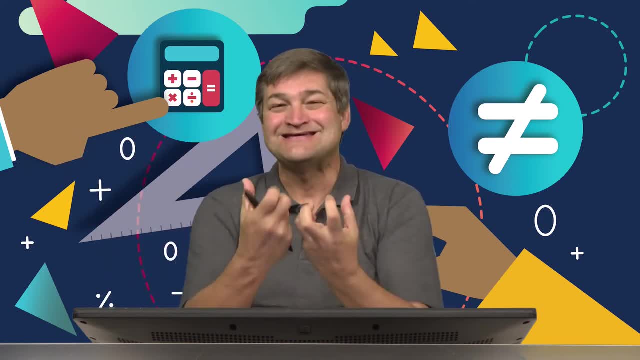 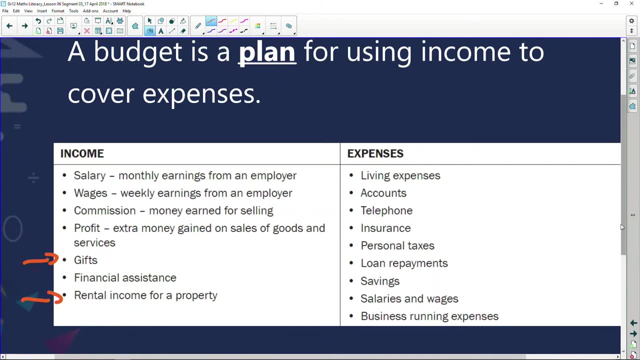 flat or your little chalet. That's money coming in Rental income for your property. Okay, Then we've got expenses, Guys. we all know what expenses are. They're living expenses, right, Like paying food, paying for food having. 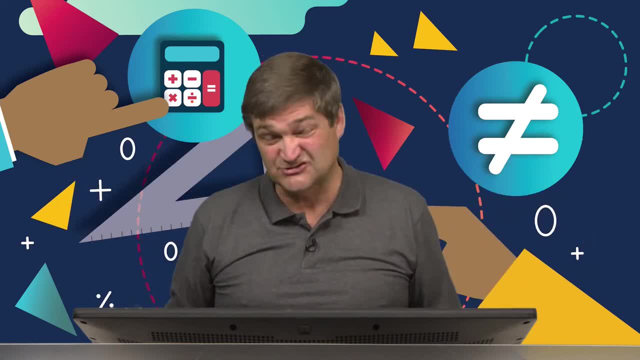 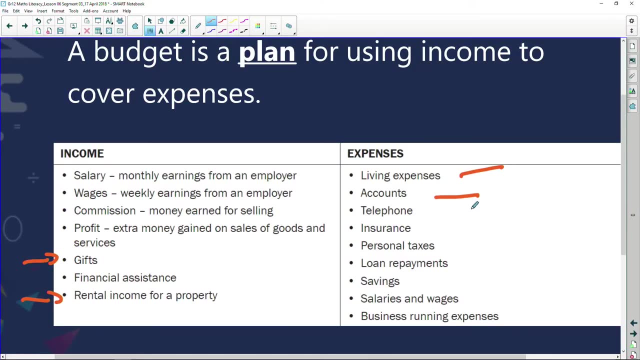 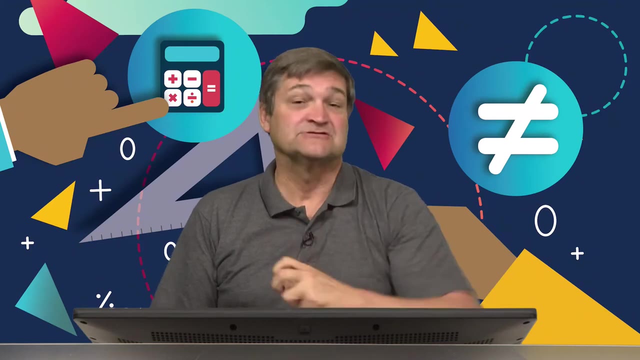 to buy clothing, All right, All those kinds of things that you got to pay to live. We also have different accounts that you might have. Like I said, you might want to go off to a metric dance, for example, You might want to buy a dress, And so you buy this address on account and every month, 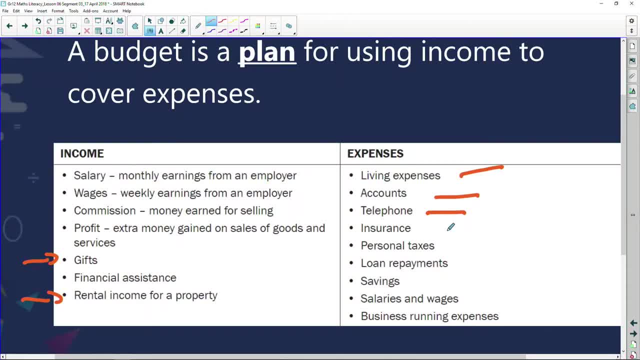 you got to pay it off. Telephone bill: We just had a session before this one looking at cell phone bills, having to pay those right Insurance. Why do we have insurance? Well, if you've got a motor car and you're involved in an accident, you want to make sure you. 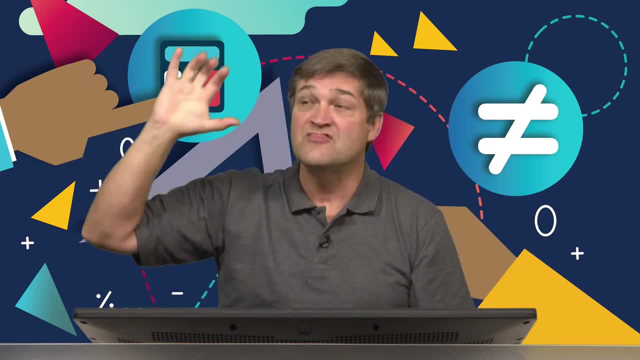 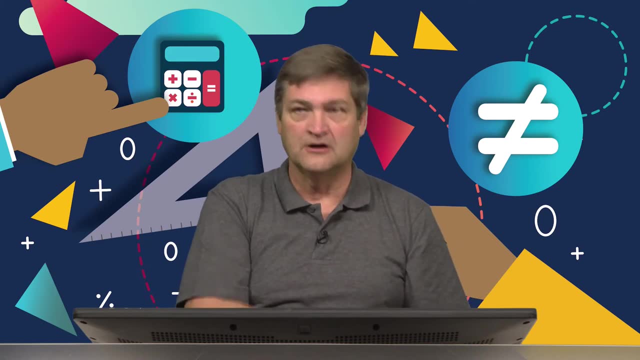 belong to a good insurance company that will pay you out and you won't have a headache of saying, Oh, now I've got to pay it off. Okay, For all these repairs for my car and the other car. Okay, Personal taxes, tax that. 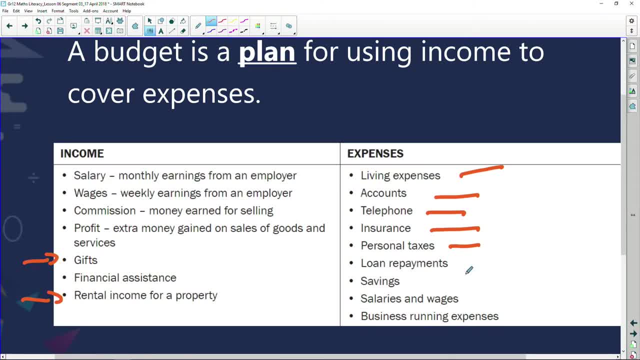 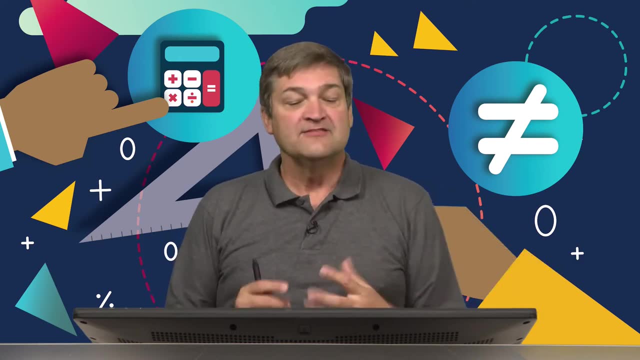 you got to pay. Those are expenses. Maybe you took out a loan and you've got to pay that back every month. Okay, Saving, You're saving money, Like I am- for my wife's birthday trip, Okay, So every month I've been putting money aside. That is still an expense, because 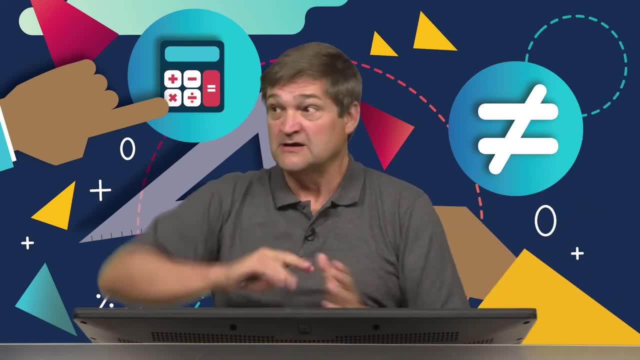 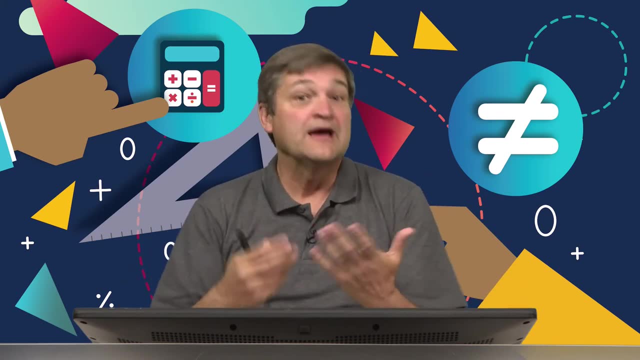 I can't pay for it. I can't live off it. It's not money coming in, It's money coming in. It's money I'm putting aside. Okay, Salaries and wages. Maybe you've got someone who works for you and you've got to pay them every month. If you've got a business, your business will. 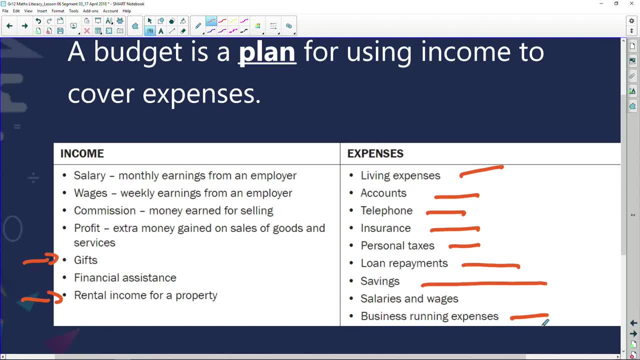 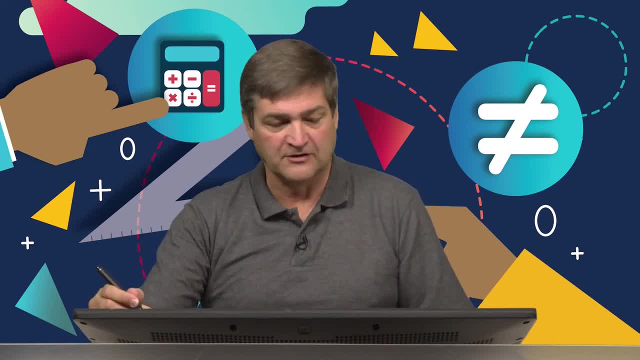 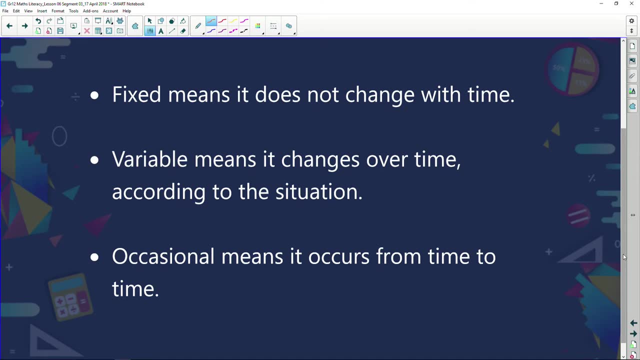 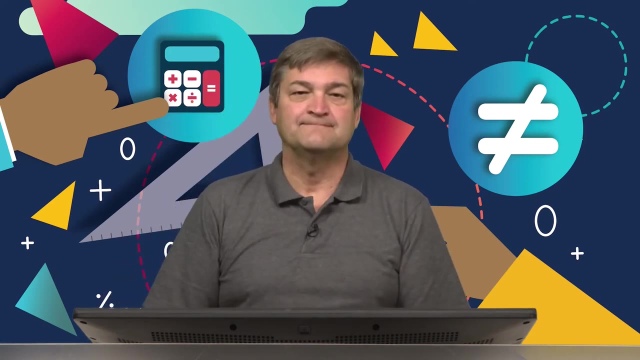 have running expenses. So we've got income and we've got expenses. When I go further, I'm going to look at the type of income or the type of expenses. Now we can have fixed income and fixed expenses, right? What does fixed mean? Fixed means it does not change with time, So I know that my salary 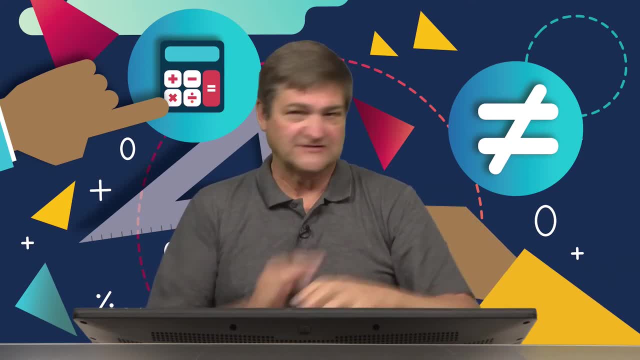 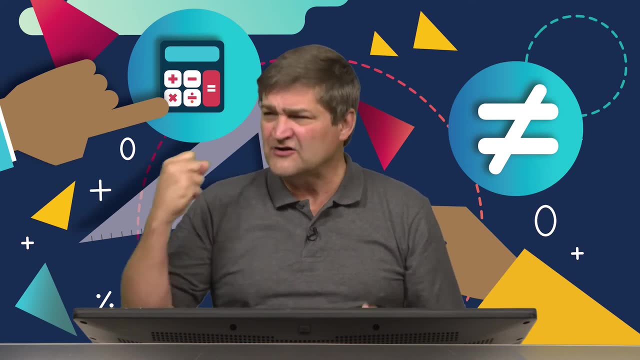 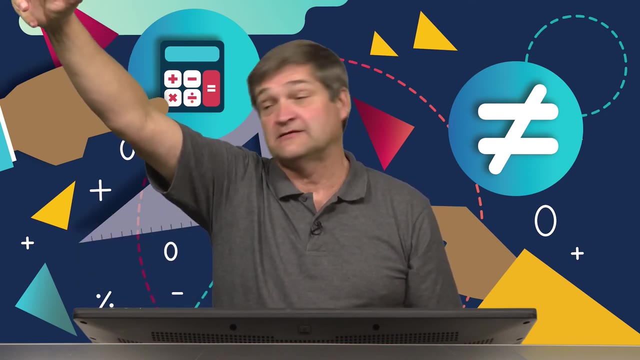 for this year is going to be so much every month. It's never going to change, It's fixed. Okay, I also have fixed expenses: My car. I've got to pay 1,400 rand every month for my car And one month I'm not going to pay 1,600 and the next month every month I'm. 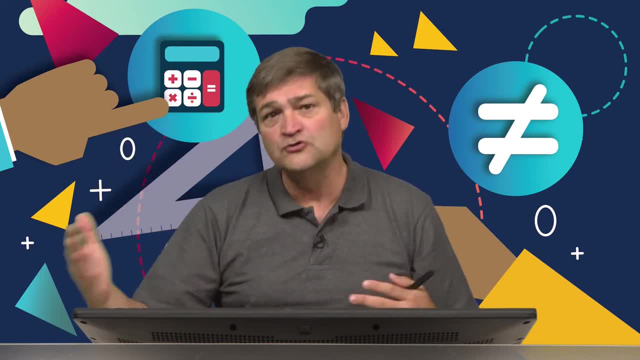 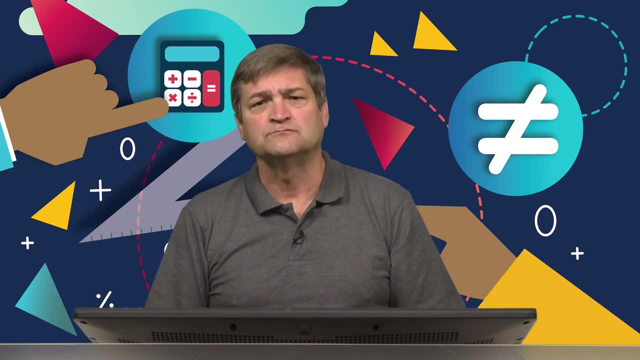 paying the same amount for my car. My rent for that whole year is going to be exactly the same, Why? Cause I agreed I will pay you 500 rand a month to live in your back bedroom. Okay, I know, every month I'm paying. 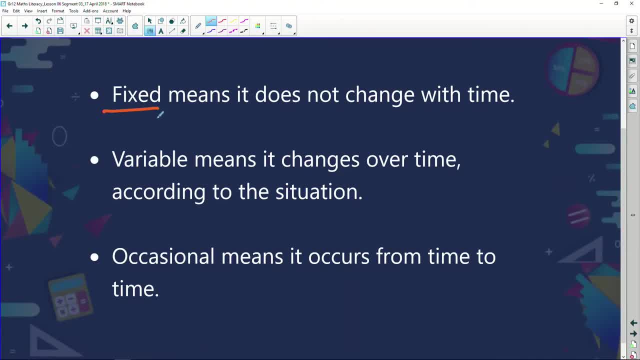 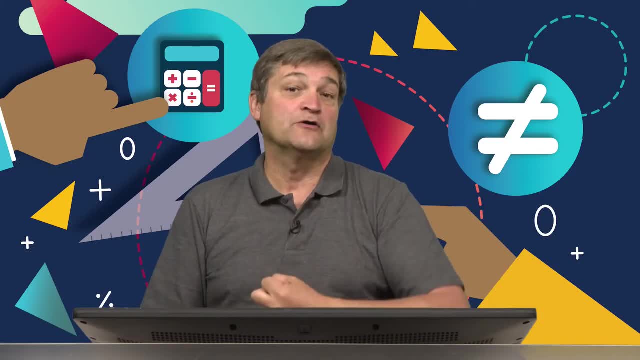 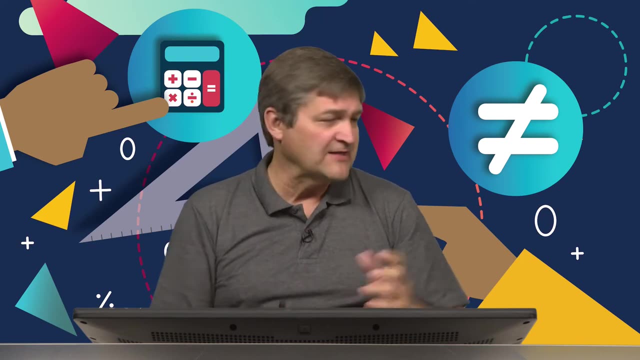 the 500 rand, Whereas variable means it changes over time according to the situation. So if I work on a commission basis, like I said, let's pretend I sell cars- I can't say at the beginning of the month This month I'm earning so much because I don't know how many cars I'm going to sell this. 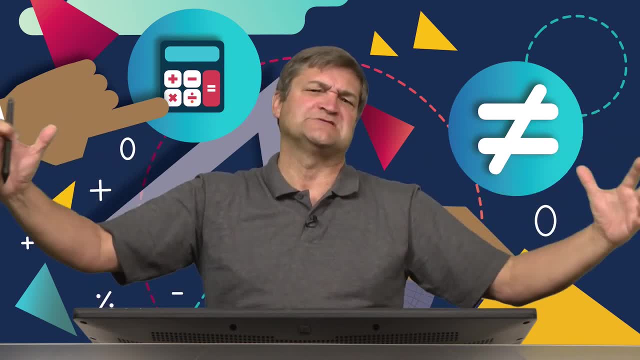 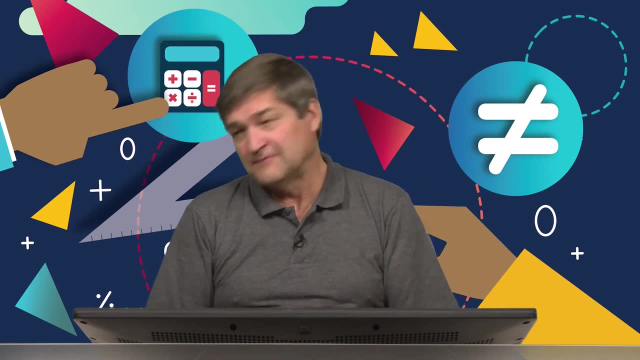 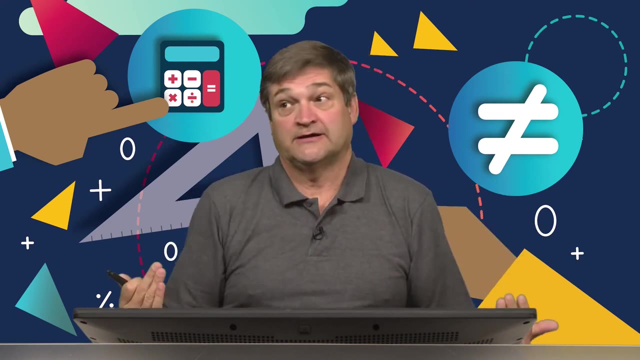 month. Okay, If I sell lots of cars, wow, big salary. Sell a little bit of cars, Oh, little salary. Okay, So I can't say at the beginning of the month, my dear, go out and spend 10,000 rand on a dress, Why, Cause? this is how much I'm earning. I actually don't. 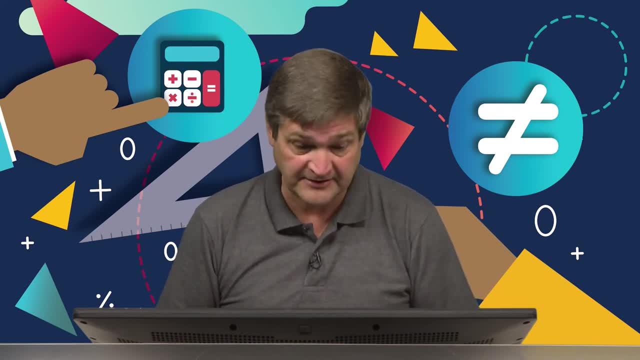 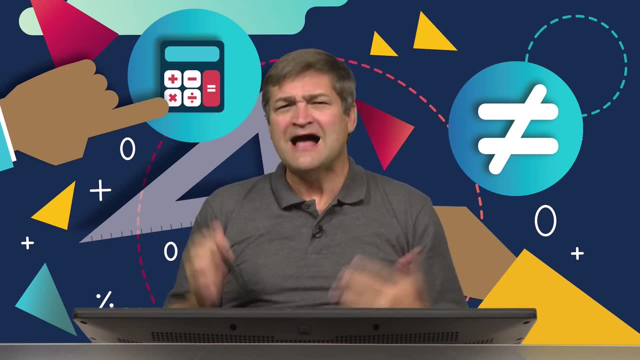 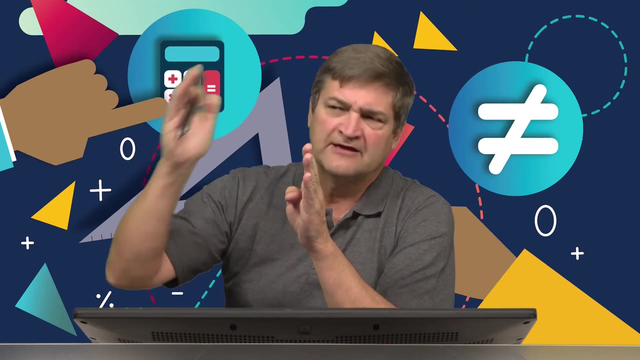 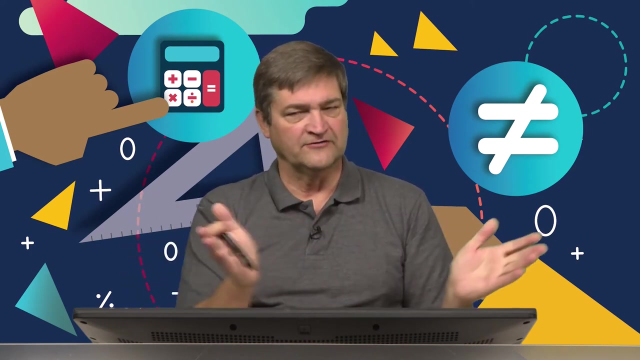 know how much I'm going to earn. All depends how many people want to buy a car that month. Variable expenses- Great. I can't tell you right now that my petrol bill this month is going to be exactly 245 rand and 16 cents. Why? Because I don't know the exact route I'm going to be following. 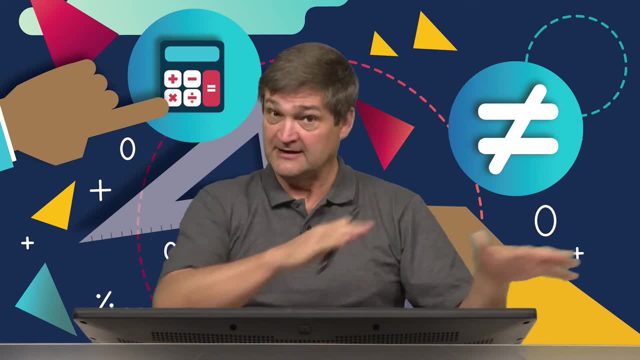 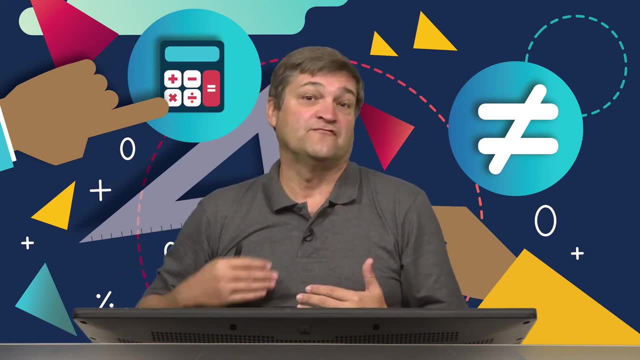 I might go decide to go for a nice little Sunday drive. Okay, I might even if I'm going to work and coming back, have to follow different route. I might go fast one day and slow it another day. there might be a lot of traffic. some stop, start, stop, start, stop. 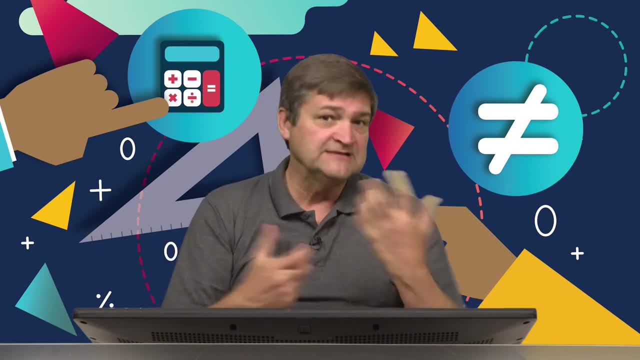 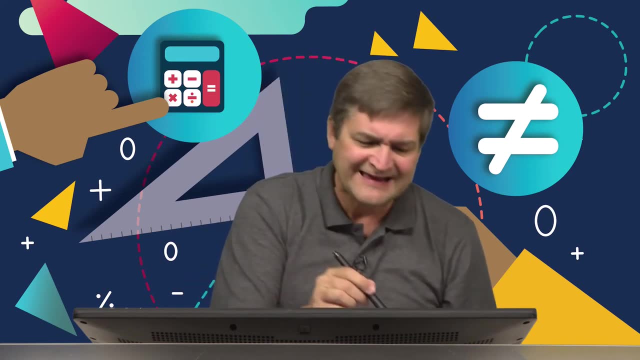 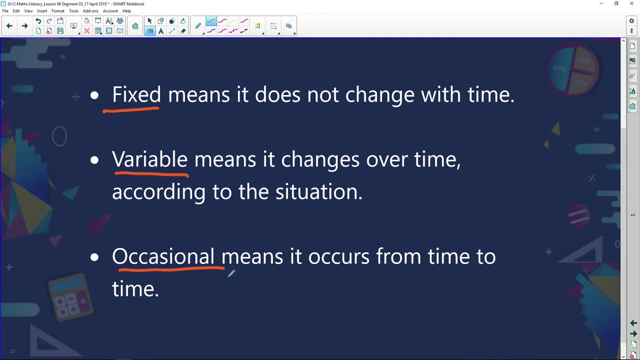 start using loads of petrol. so variable means it's going to change. you know it's going to be there, but you don't quite know what it's going to be every month. then occasional means it occurs from time to time. okay, so maybe at the end of 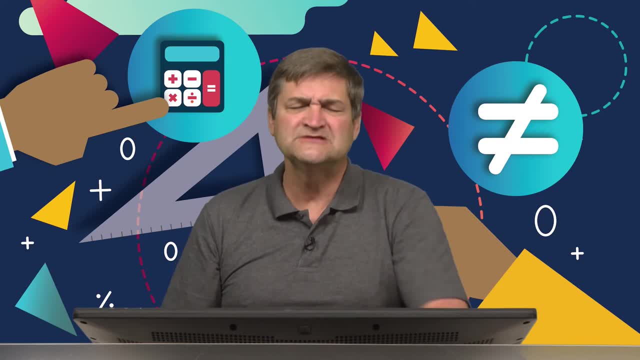 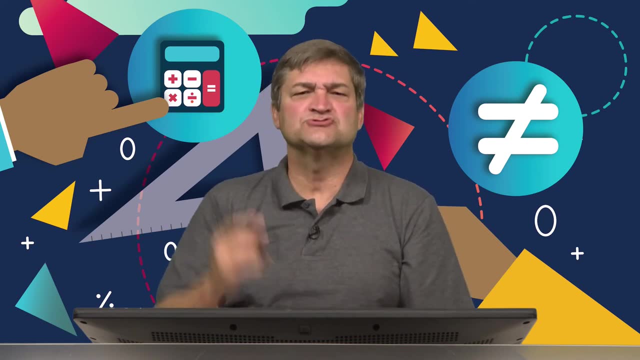 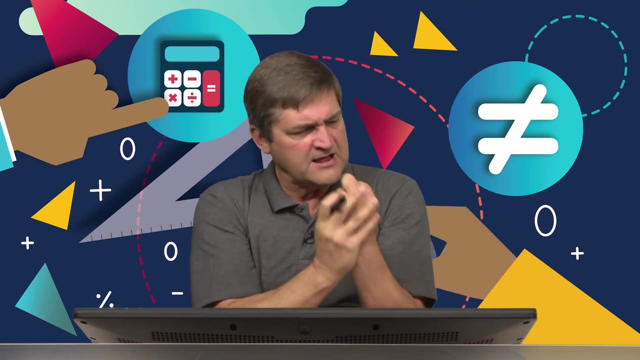 November my boss comes to me and says: you know what, Pete, you've been a fantastic teacher this year. I'm gonna give you a little bonus: here's an extra ten rain. you go and buy yourself a chocolate. okay, then I'm gonna say: cool, that is money coming in. it doesn't happen every month. it doesn't happen. 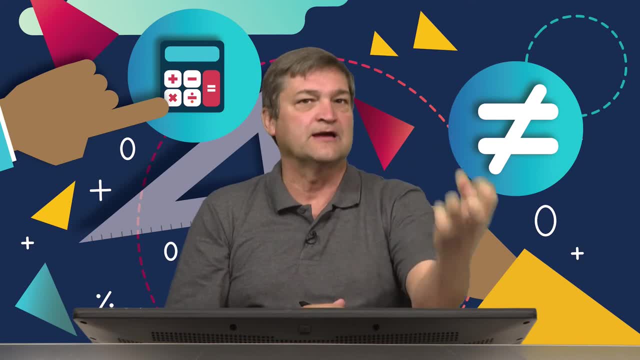 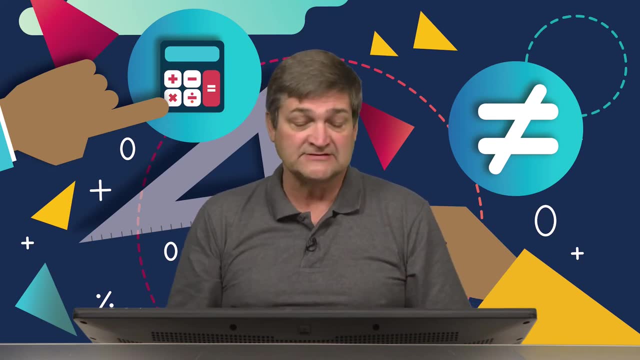 every year, but on the occasion I get an extra little bit of money coming in, or you might am submit your taxes and the tax man says: you know, mr Timpson, we so sorry, we've got a little bit of money coming in and I'm going to give you a. 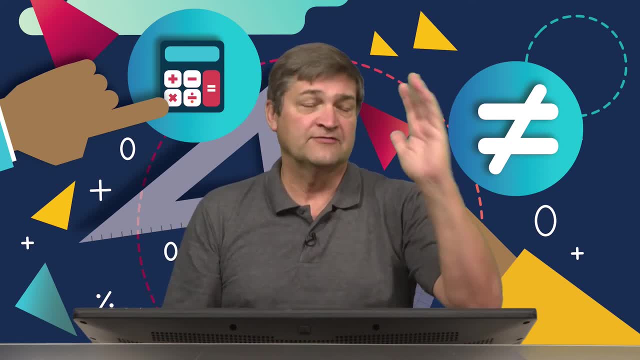 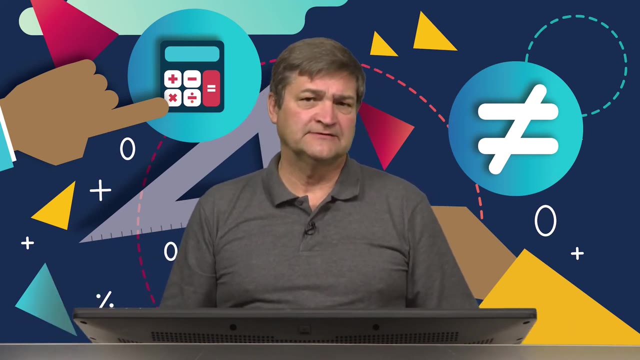 little bit of money every month, but it's not something I'm doing getting every month. occasional expense might be, for example, suddenly your car breaks down, okay, and the engine burns out, or something weird happens. the car goes into the garage and the guy says: listen, sir, you now owe us 4,300. rank that is an. 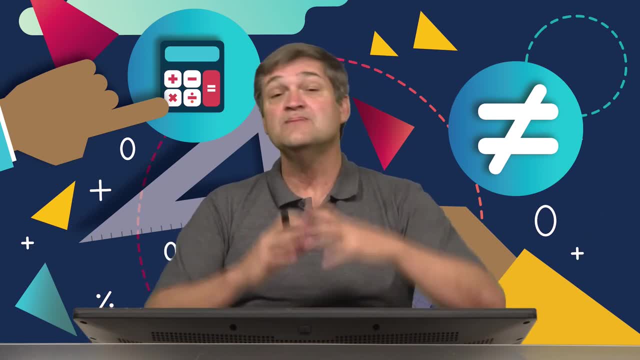 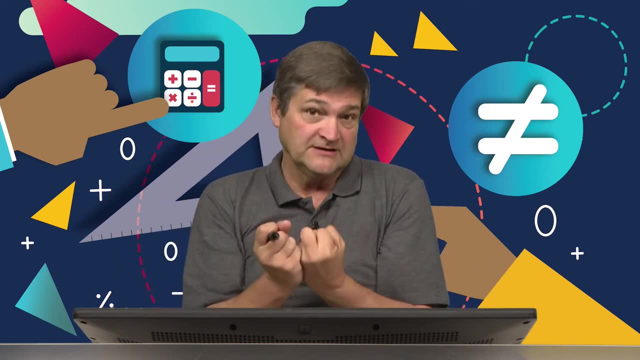 an occasional expense. It doesn't happen every month, but on the odd occasion something goes wrong with my car and I've got to pay it. I don't know what that expense is. I don't know what that income is. It comes in or I've got to pay out on the odd occasion. Do we understand the difference? 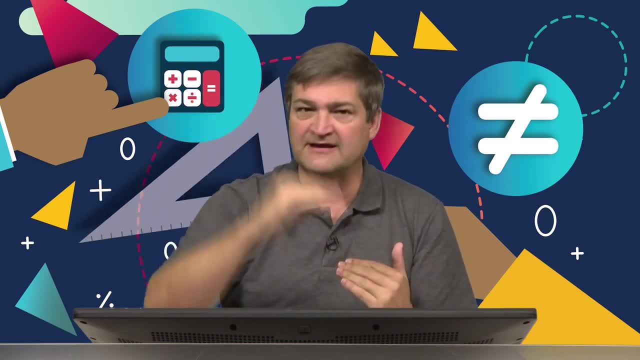 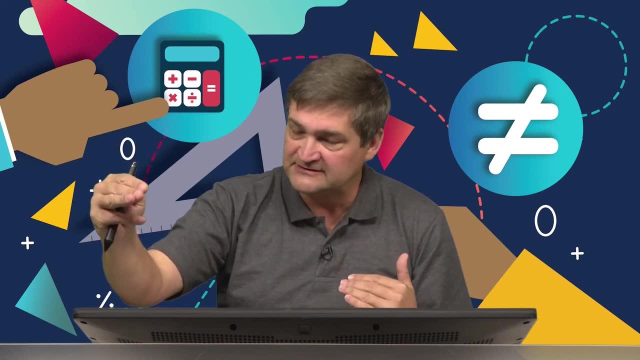 So fixed means I know what it's going to be and it's going to be that every month. Variable means I know I'm getting money in but I can't tell you how much. or I know I'm going to pay this at the 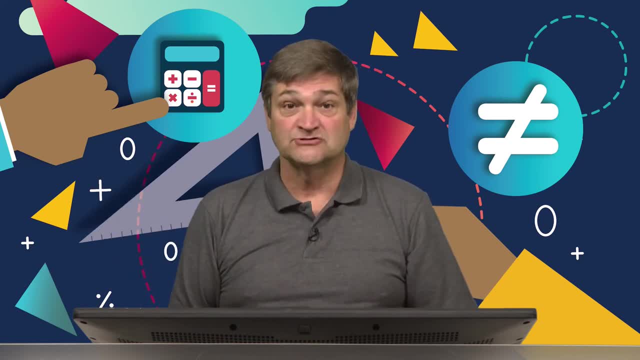 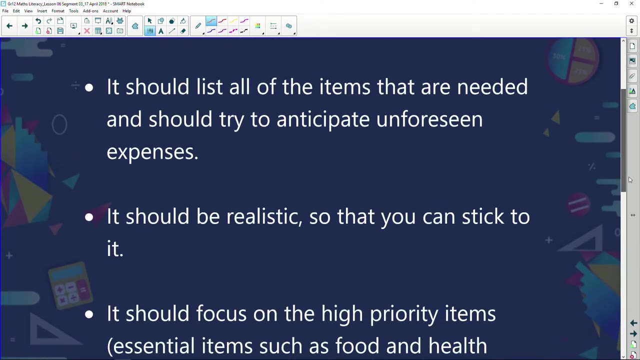 end of the month, but I don't actually know the exact figure, And occasional means voila, on the odd occasion I get money coming in. Okay, so let's have a look here. There are several things you should aim for in your personal budget. It should list all the items that are needed and should try. 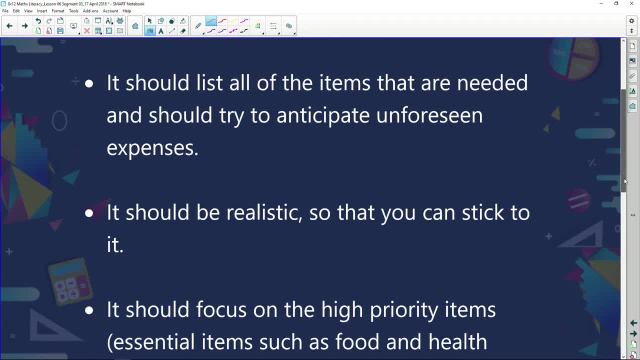 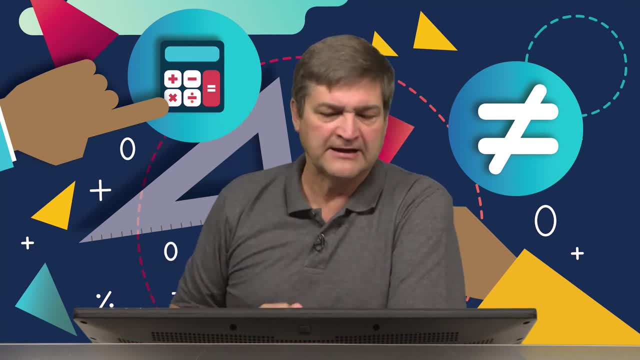 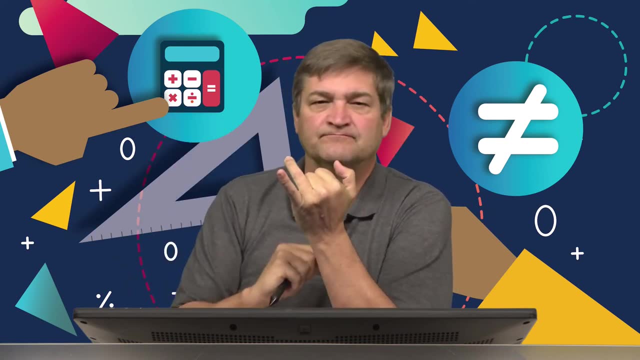 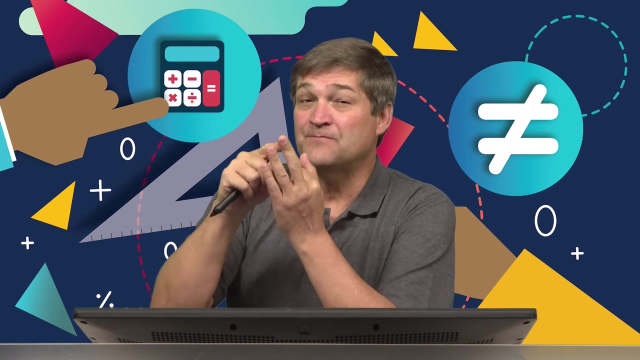 to anticipate unforeseen expenses. So, just checking for my wife With this story, I'm planning. I know I've got to plan the price of the train ticket to Cape Town, I've got to plan the price of the accommodation, Okay, And I've got to plan the price of coming back by the aeroplane. But 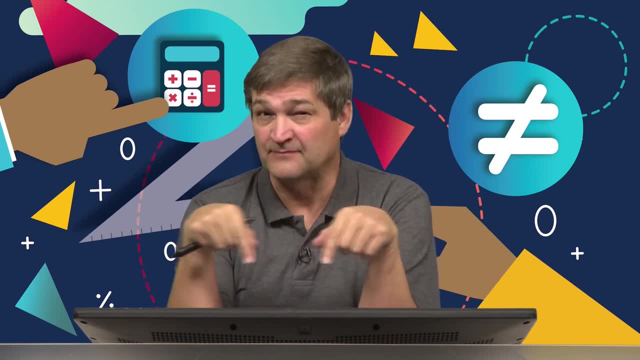 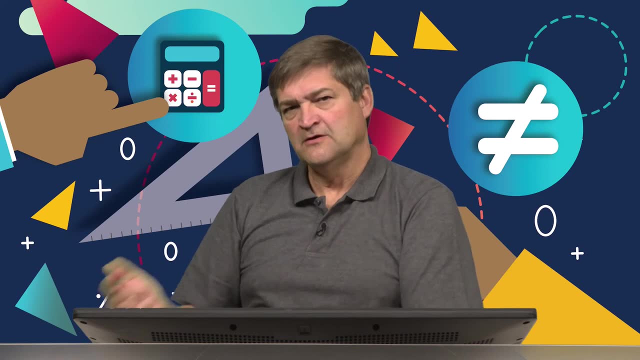 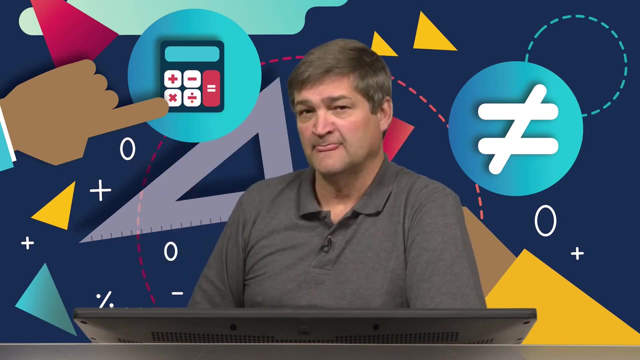 there are other things that might happen that I'm not aware of, Okay. So, for example, here's something I never thought of: When I go, I park my car at the train station. Guys, that's going to cost me money every day that it's parked there. 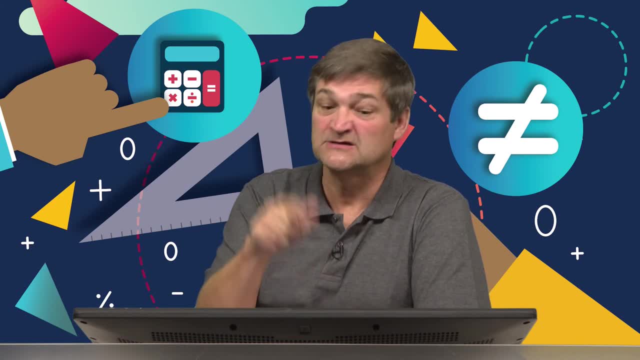 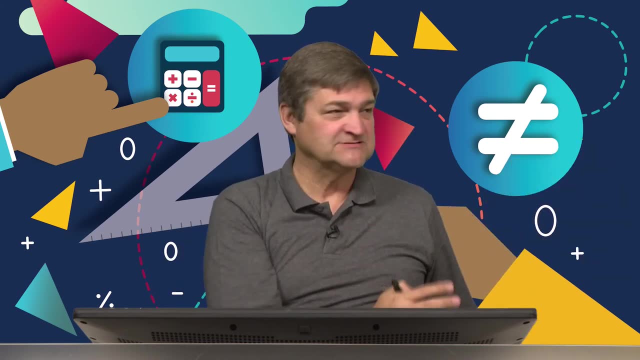 Ish, forgot about that Unforeseen expense. Got to take that into account. Okay, When we get there, my wife might see a fantastic dress and say: oh, it is my birthday and this whole trip is for my birthday. I think I should also have that dress. 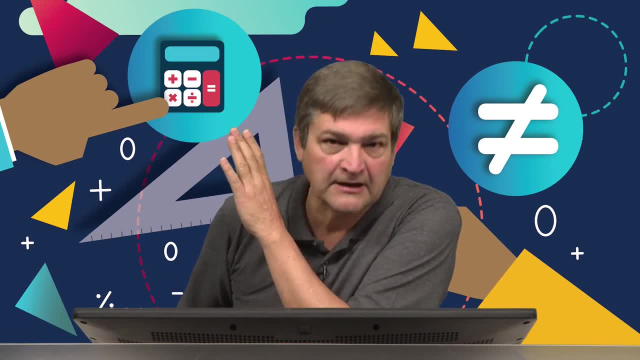 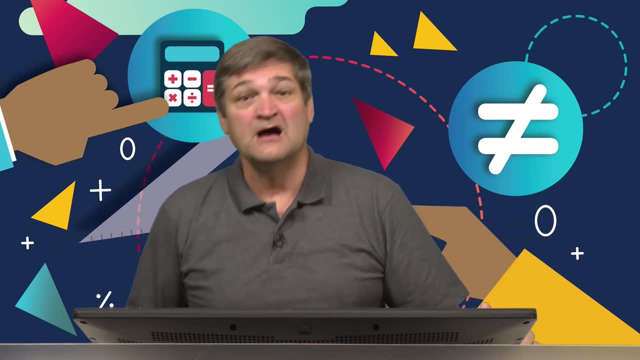 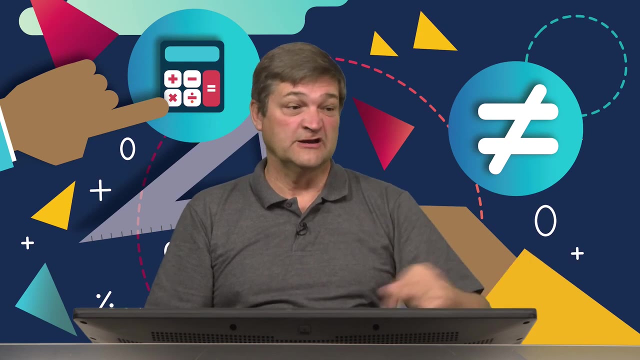 Unforeseen expense coming up. All right, Here's a worse thing, And heaven forbid that that should happen. Maybe I'm walking along, kicked my toe, it gets totally mashed against the pavement. got to go to the clinic. 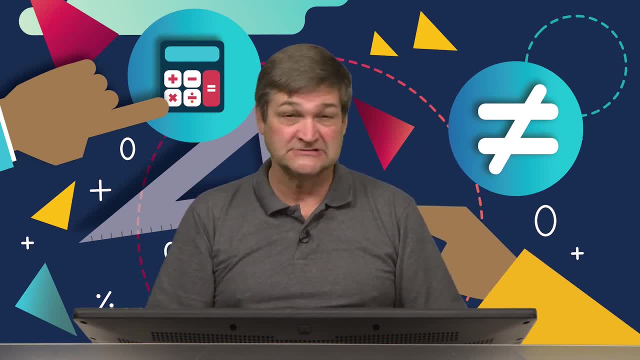 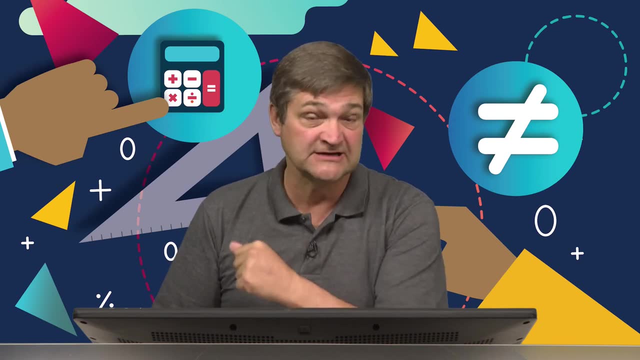 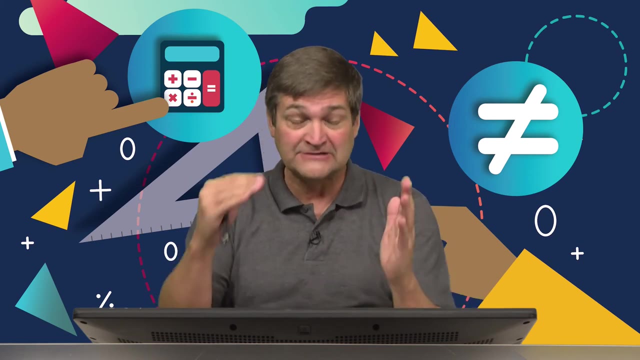 they got to fix it up And suddenly they say, sir, for that little ten minutes, that we, you, you owe us 3,400, right Unforeseen circumstance. So all these things need to be taken into account. In fact, when your parents plan their budget every month, they should say: let's. 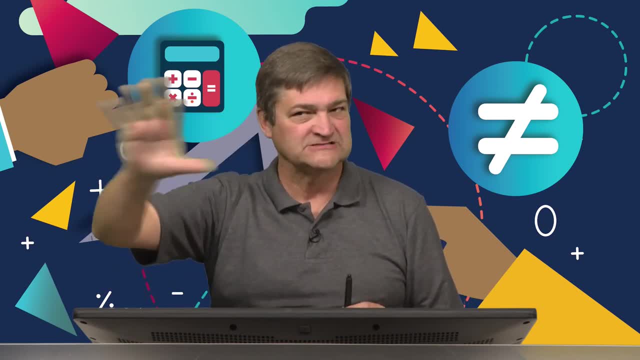 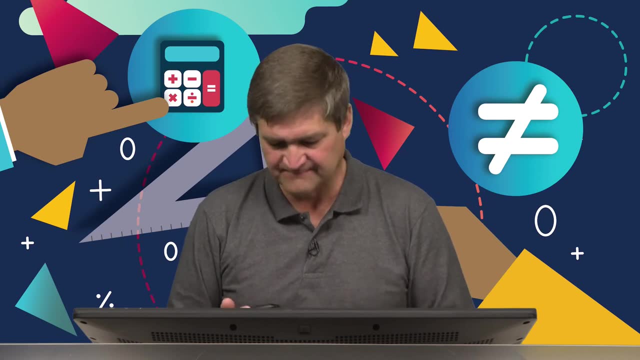 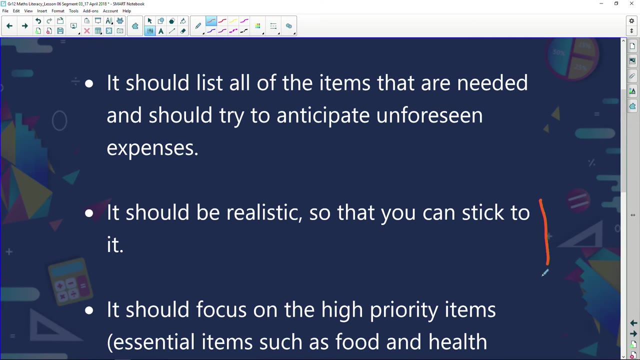 keep money aside, just for in case something goes wrong. We hope nothing goes wrong, but in case something goes wrong, let's keep money aside. okay, It should be realistic so that you can stick to it. So I'm not going to say: you know what we're getting on a train. 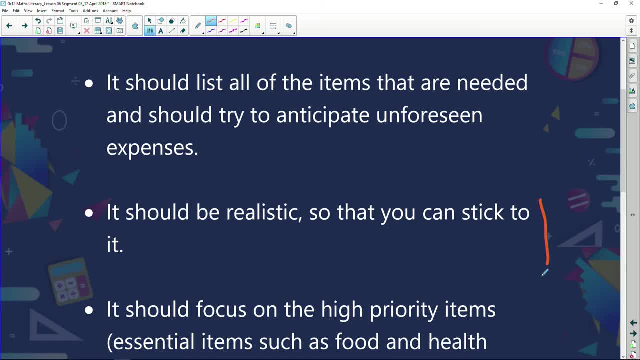 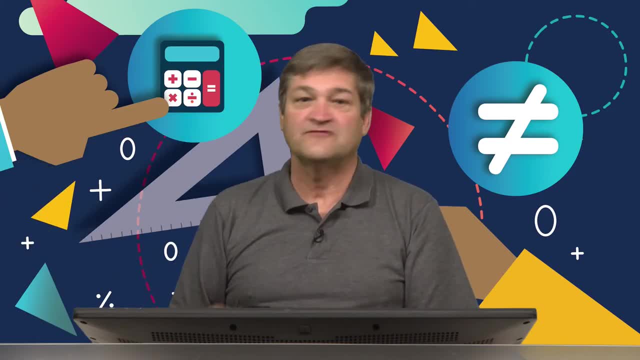 and it's going to cost me five red. And then, when we get there, we're going to live in accommodation, and that's going to cost me another five red. Then we're going to get on an airplane and we're going to fly back, and that's going to be another five Guys. 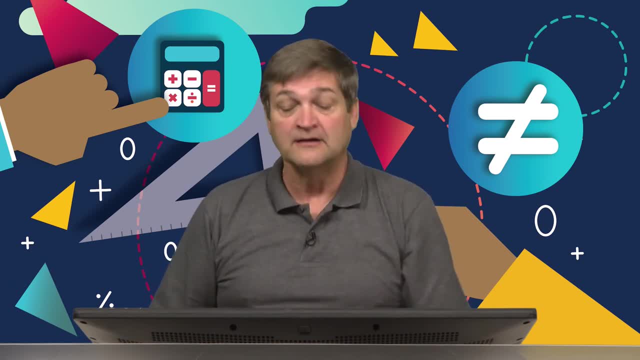 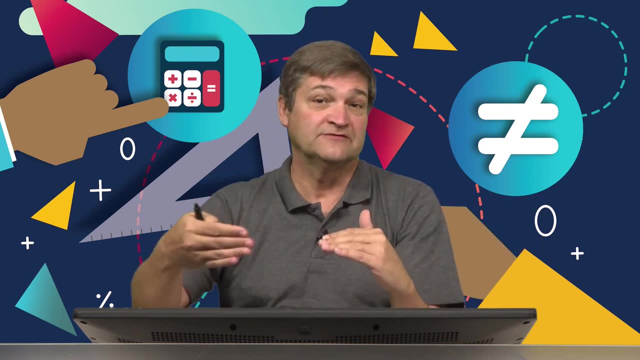 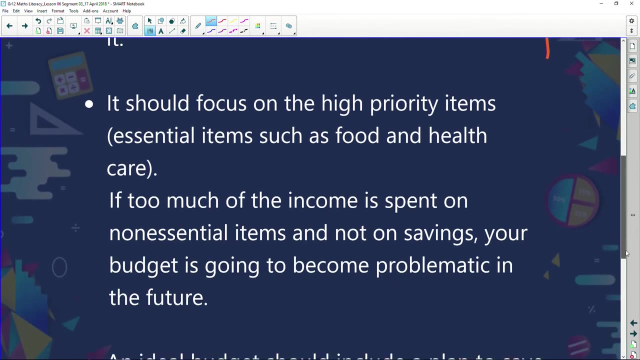 it's going to cost me a heck of a lot more than five rand. okay, So be realistic with your budget, because if you're not realistic, you're not going to be able to live by it or stick to it. okay, It should focus on high priority items, essential items such as food and healthcare. If too. 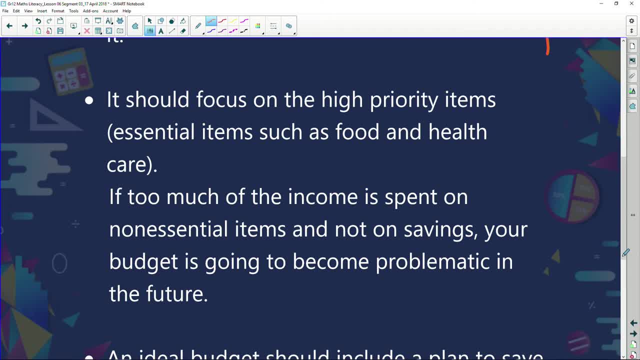 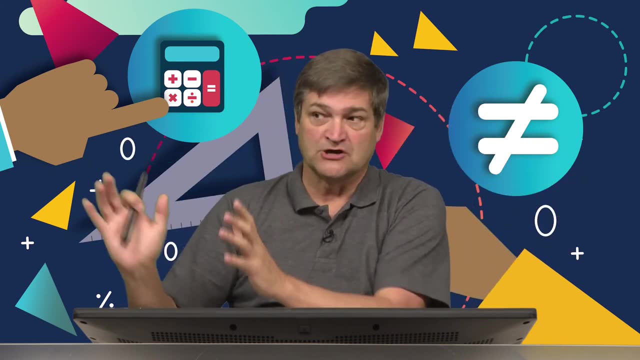 much of the income is spent on non-essential items and not on savings. your budget is going to become problematic in the future. okay, So I walk down the shop or in a shopping center, I walk past the shop and there it is. okay, The shirt. I've always wanted. The. 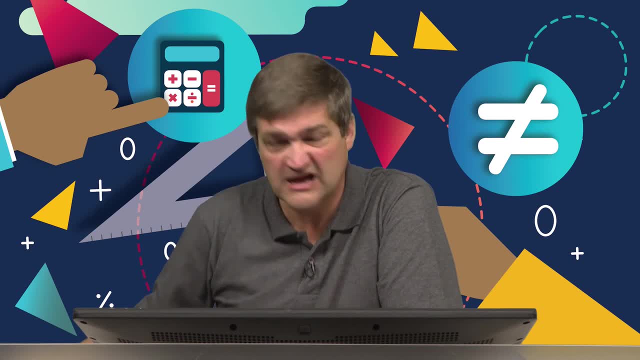 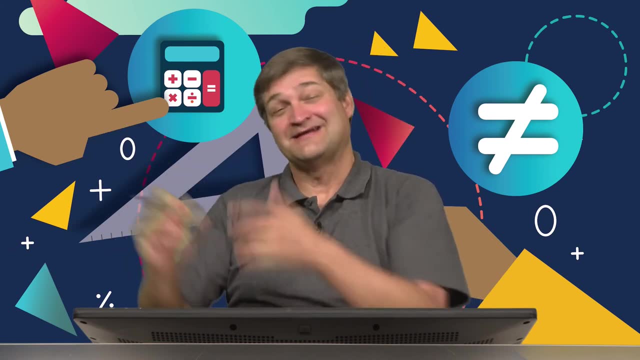 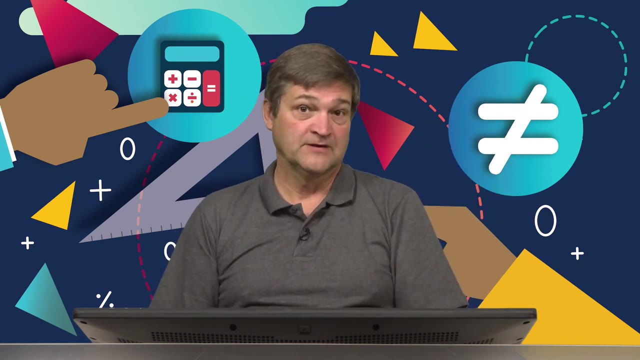 shirt I've always wanted, But it cost five hundred rand, And I never spend five hundred rand on a shirt. I think it's crazy, But I've got to have that shirt, And so I go in and I buy the shirt. okay, Then I keep going, and now I get to the shop that sells the food. 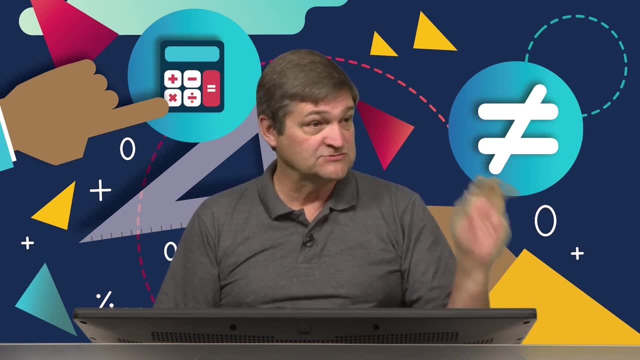 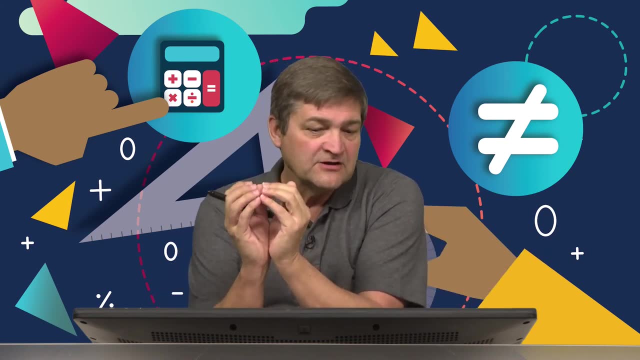 And I go in and I say, okay, we need bread, we need milk, we need this, we need that, and suddenly realize I don't have the money. okay, What's happened? I've focused on things that are non-essential. 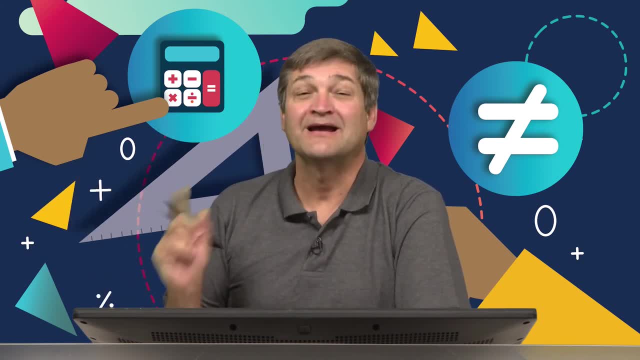 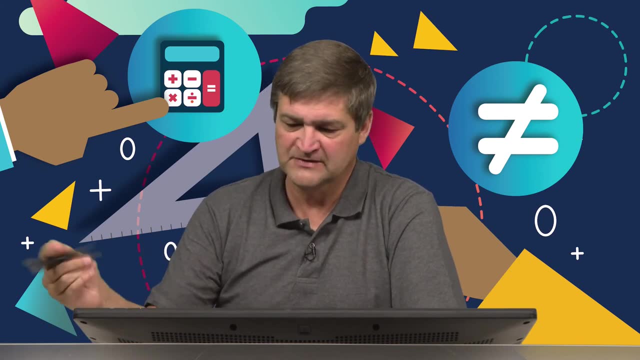 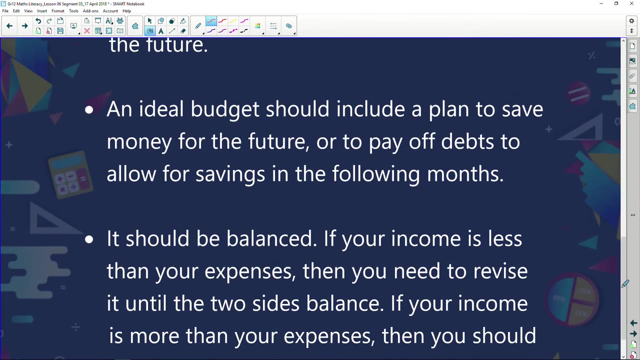 In other words, I didn't really need that shirt but I bought it anyway, Whereas I actually did need the bread and milk and should have bought that first. okay, An ideal budget should include a plan to save money for the future or to pay off debts to. 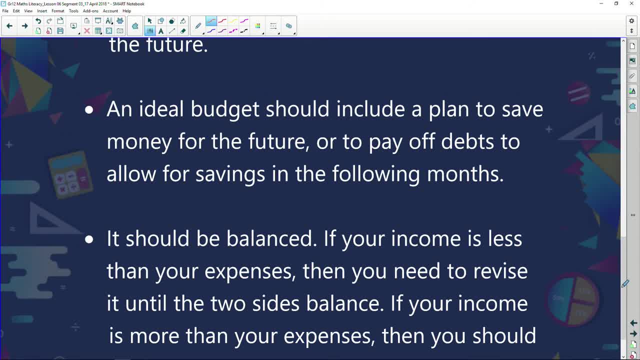 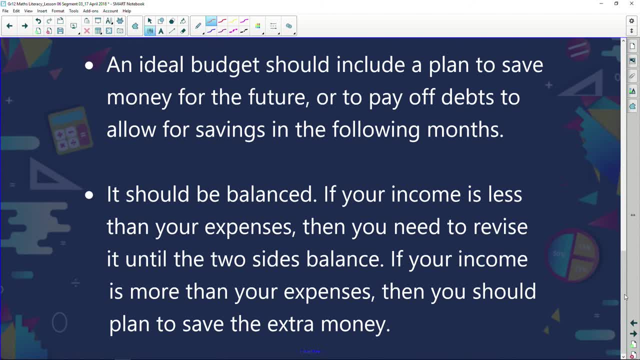 allow for savings in the following month. It should be balanced. If your income is less than your expenses, then you need to revise it Until the two sides meet, Until the two sides balance. If your income is more than your expenses, then you should. 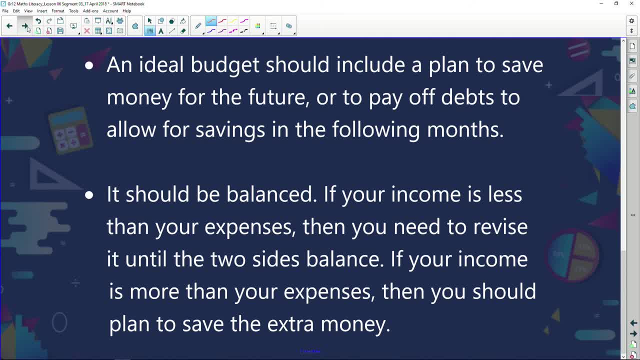 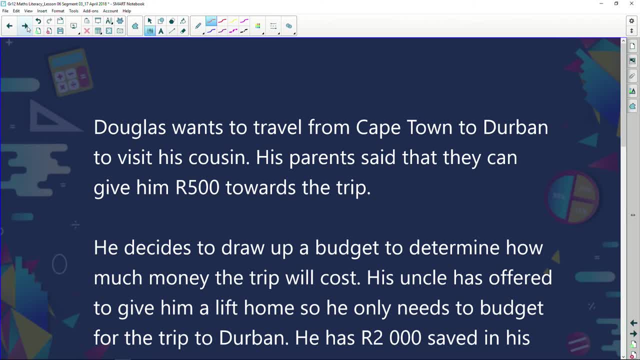 plan to save the extra money. All right, we're going to look at an example here. We don't have a lot of time, so let's just skim through it. Douglas wants to travel from Cape Town to Durban to visit his cousin. His parents said: 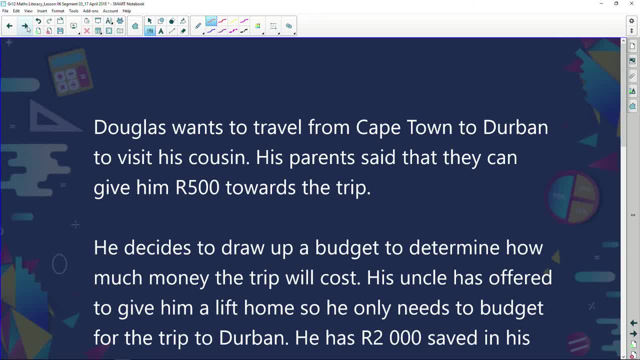 that they can give him five hundred rand towards a trip. He decides to draw up a budget to determine how much money the trip will cost. His uncle lives in a big house, so he only needs to budget for the trip to Durban. He has saved. 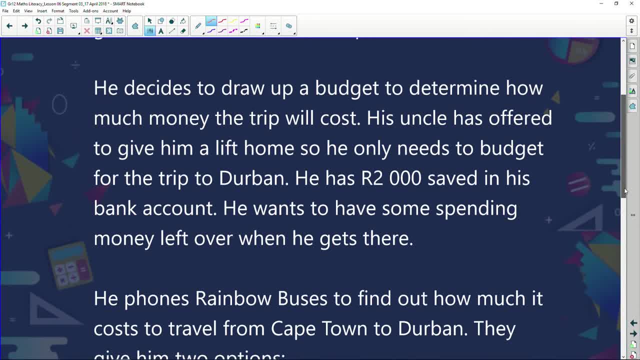 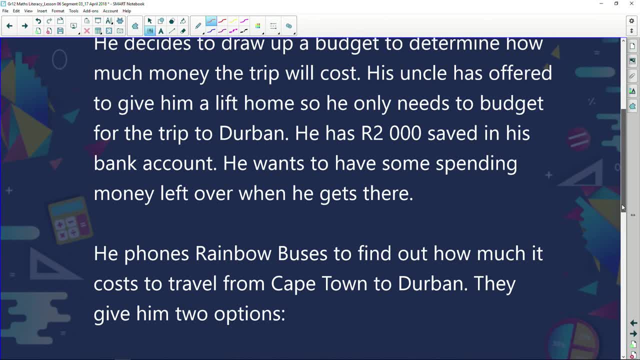 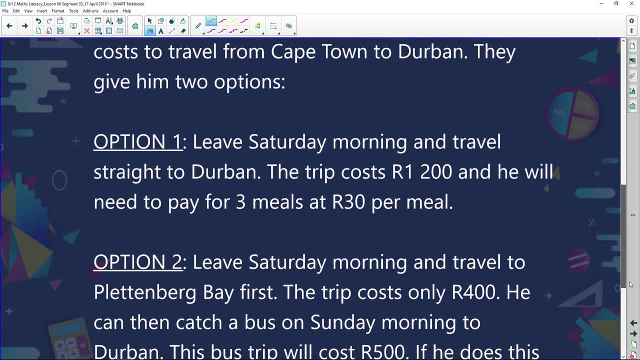 two thousand rand saved in his bank account. He wants to have some spending money left over when he gets there. He phones Rainbow buses to find out how much it'll cost to travel from Cape Town to Durban, And they give him two options. Option one: Leave Saturday morning and travel straight. 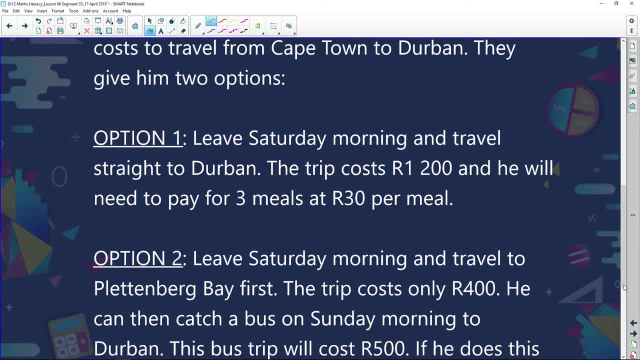 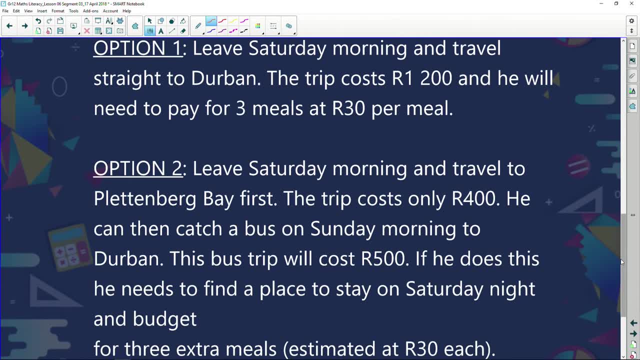 to Durban. The trip costs one thousand two hundred rand and he will need to pay for three meals at 30 rand per meal. Option two: leave Saturday morning and travel to Plettenberg Bay first. The trip only cost 400 rand. He can then catch a bus on Sunday morning to Durban. 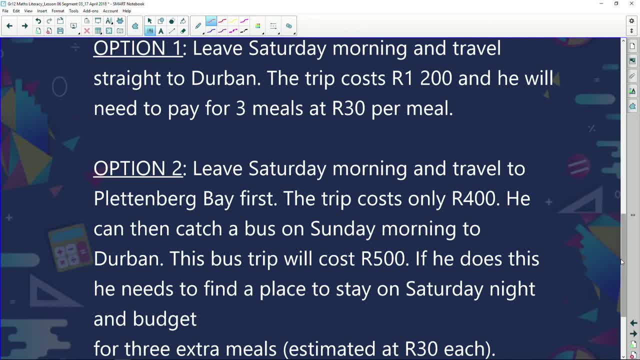 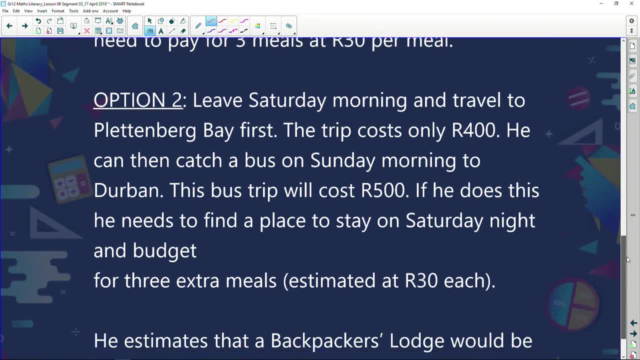 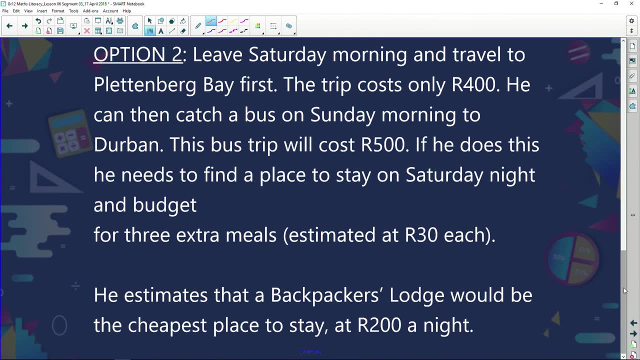 This trip will cost 500 rand. If he does this, though, he needs to find a place to stay on Saturday night and budget for three extra meals, estimated at 30 rand each. He estimates that a backpacker's lodge would be the cheapest place to stay, at 200 rand a night. Right, so now let's. 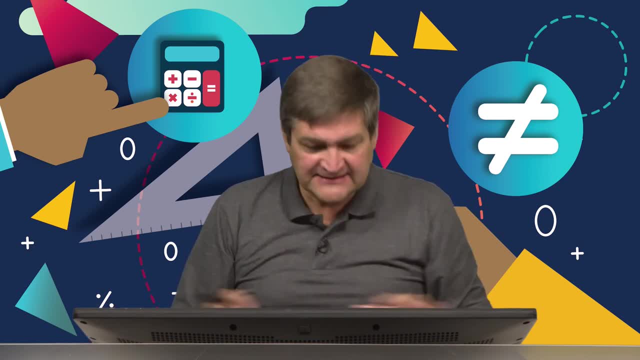 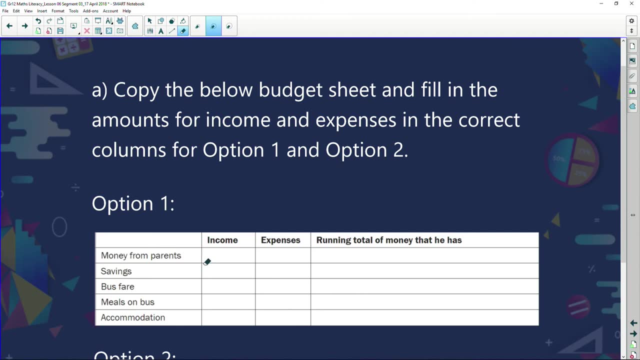 quickly draw a budget for Douglas. Let's have a look here. There's income. there's expenses- Money from parents. he got 500 rand. What is that? That's income towards his holiday. Okay, so let's write that down straight away. He's got 500 rand. He's got savings of 2,000 rand. That's income towards. 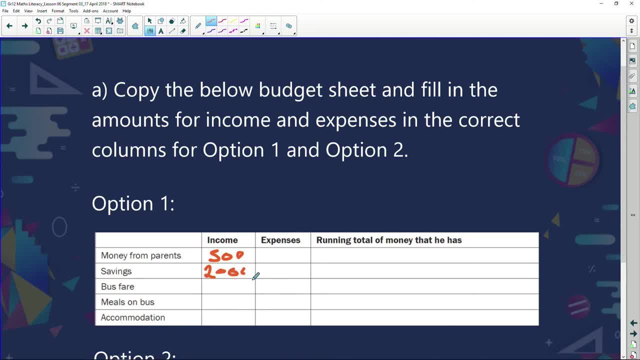 his holiday, isn't it? He's got 2,000 rand Bus fare. The bus fare was 1,200 rand- Meals on the bus, and that's an expense, eh, folk Meals on the bus. He'd had to pay for three meals at 30 rand each. That is 90. 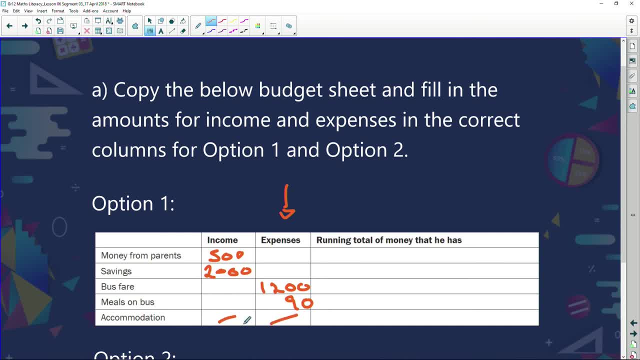 rand. Accommodation's not going to cost him anything. Why? Because he's going on a bus straight to Durban, uncle paying for the accommodation. Total running of the money has He has 500 rand. He adds another 2,000.. He's now got 2,500 rand. He then has an expense of 1,200. 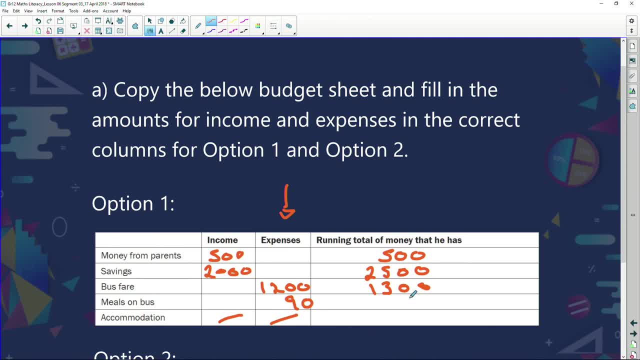 So he's left with 1,300 rand. Another expense of 90 rand, So he's left with 1,210 rand. That's how much money he's left with. With option two, it was a little bit different. He still had the income of. 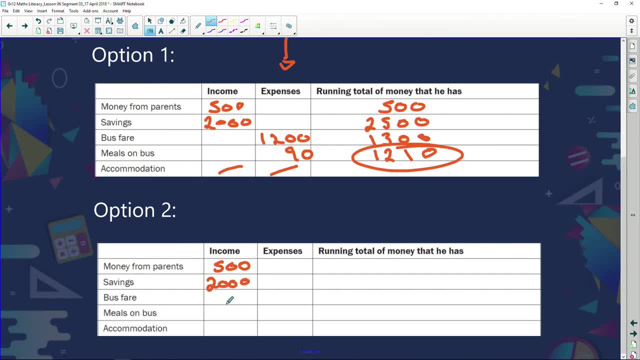 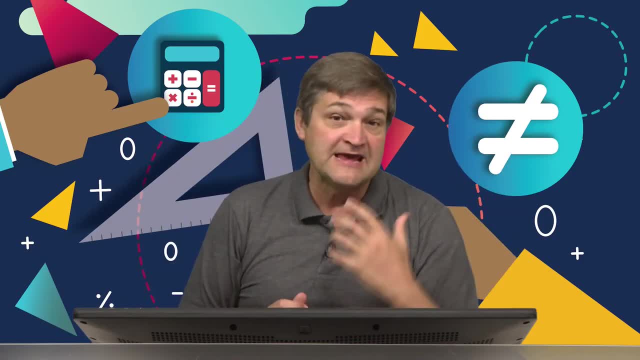 500.. He had the income of 2,000. But remember, his bus fare was slightly different. He paid 500 and 400 rand, which came to a total of 900. But then he had to pay for extra three meals and he had to. 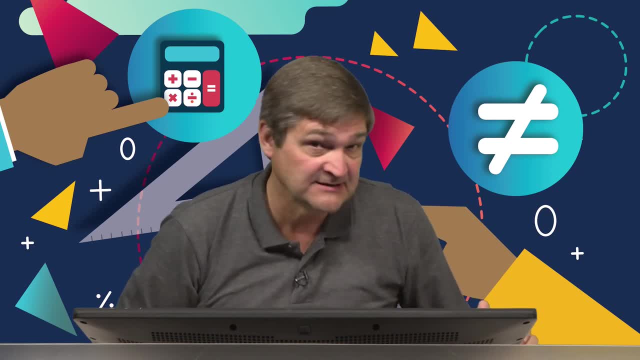 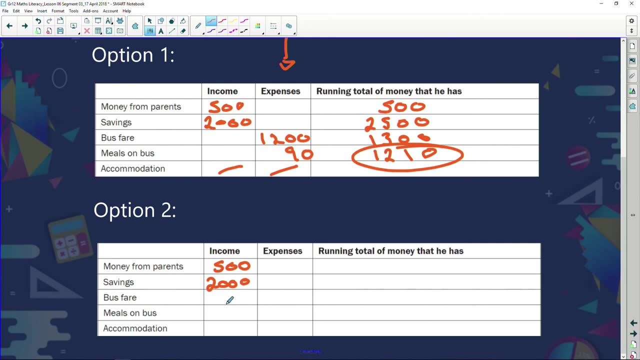 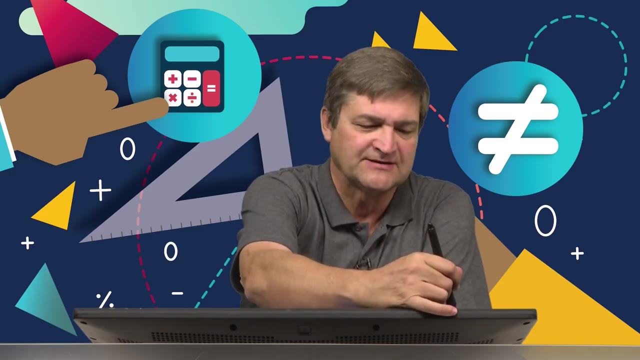 pay for accommodation because he was stopping over at Plettenberg Bay. But that's basically how Douglas has had to work out the budget And then he works out which would be the better option with him. We've run out of time, So let's just summarize this very quickly, And we're going to say the following In summary: in the segment we've